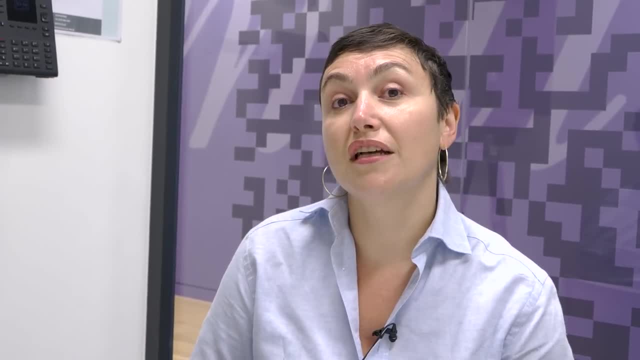 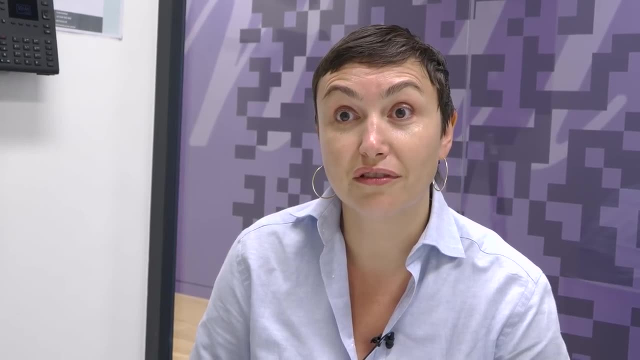 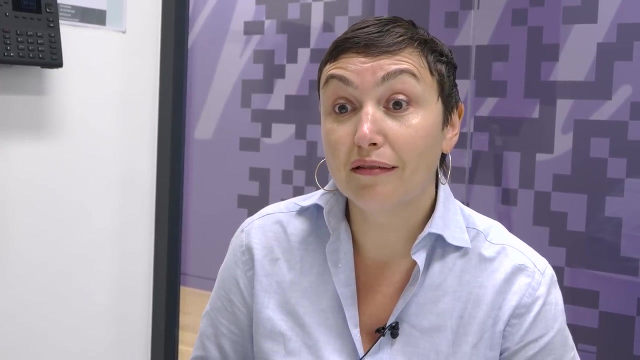 because it's still a building. but perhaps it will not tell me anything about any University departments, because National Theatre is not a university or it's not a location for a University, right? So how does Google know about the world around us, about London? Well, because it uses the knowledge. 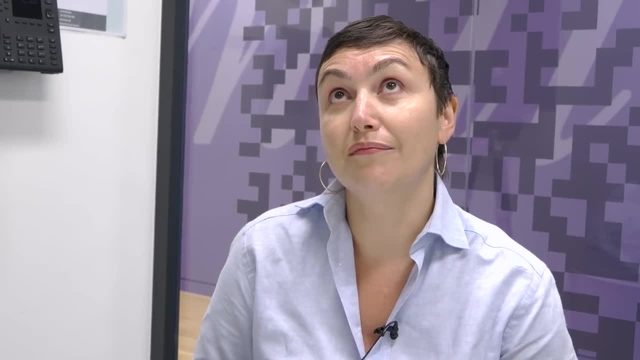 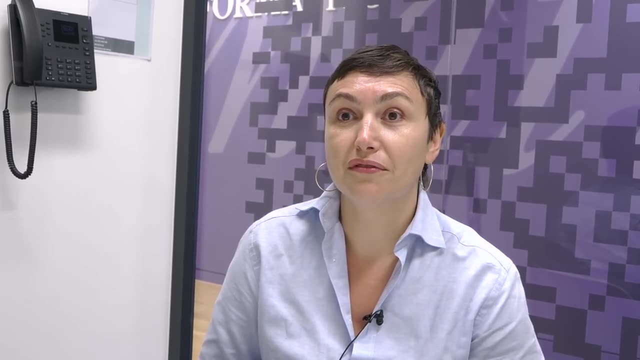 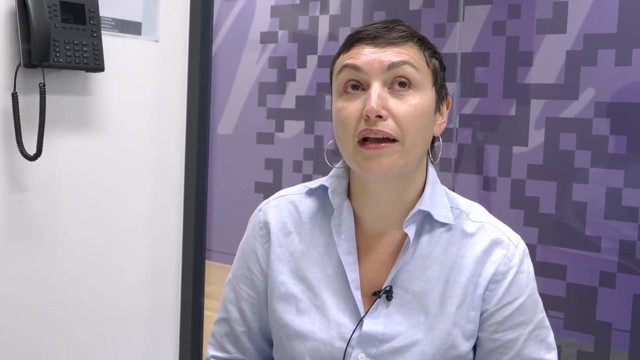 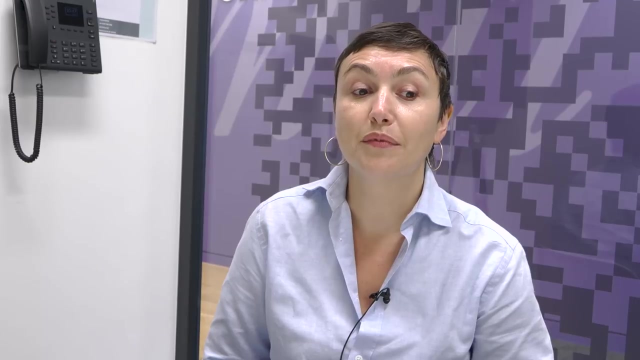 kernel- And I say the because actually Google is the company that has coined this term- But actually the principles and the technologies have been around for much, much longer, in fact decades and decades- where AI researchers were building so-called knowledge bases, which are very similar types of IT. 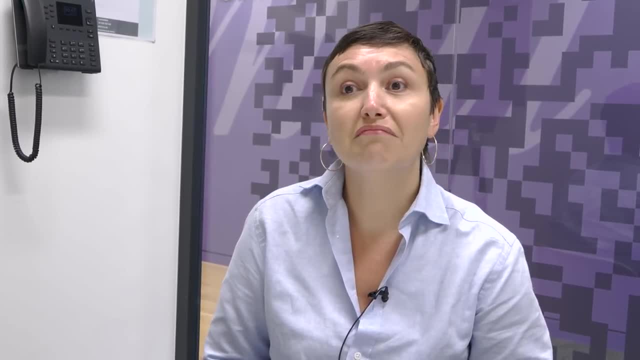 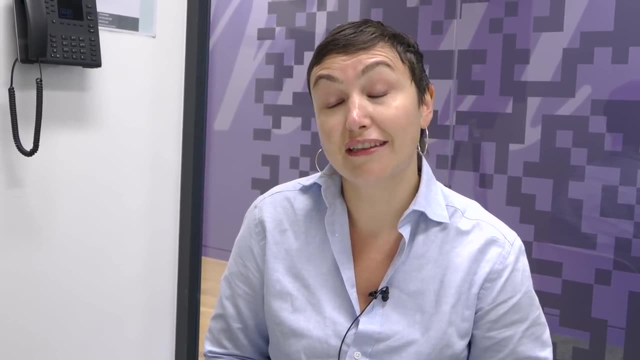 systems that are encoding knowledge, information, data. I don't think we need to go into a big discussion about what these three mean and how they are different from each other. They are, In this case, in the example I had it's. 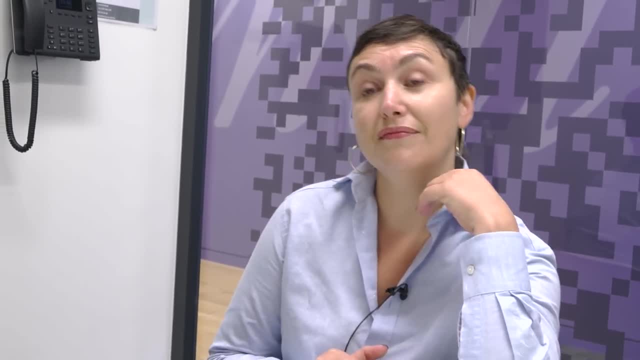 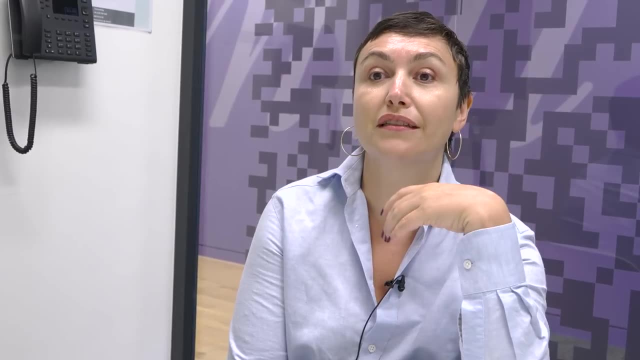 about knowledge about London. What connects all these different pieces of data together? So this is the knowledge graph. This is the knowledge graph And the knowledge graph as it is today, not just in the case of Google, but pretty much any large organisation that then provides this sort of internet. 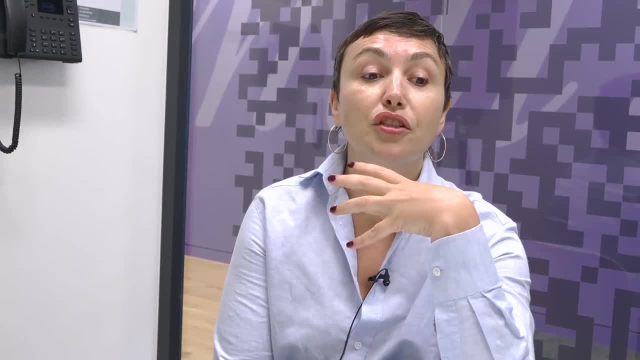 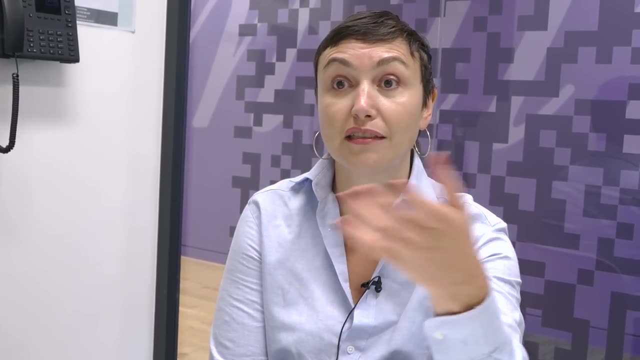 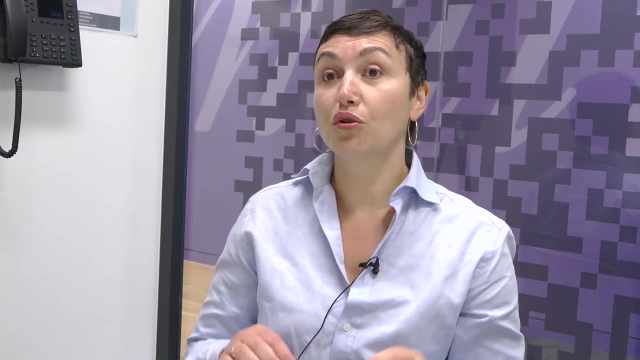 information services has one. They are huge databases with billions and billions of facts like this: Bush House is located in London at this address, And this information is extracted from documents, say on the King's website. somewhere there is information about Bush House and it's written: 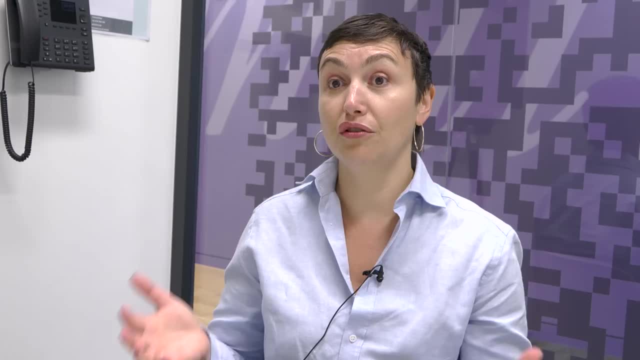 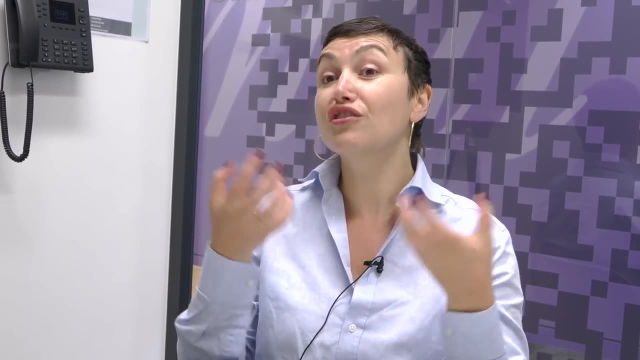 appropriately. To finish, this is written publicly. This is a document you have to, probably in text- and Google has the machinery to process all this text and recognize that this string bush house is probably a building- and learn that information, that structured information, and store that in their knowledge graph. 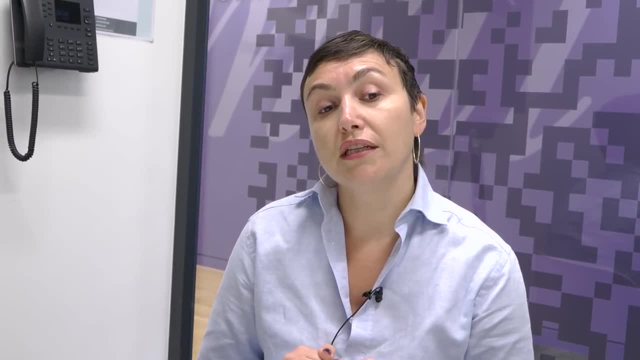 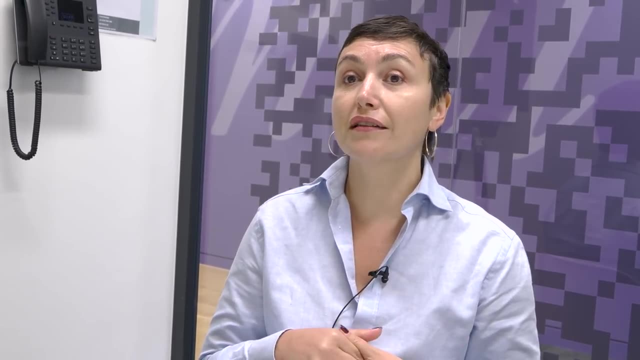 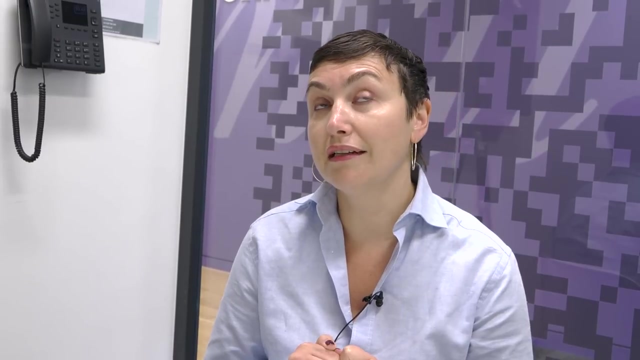 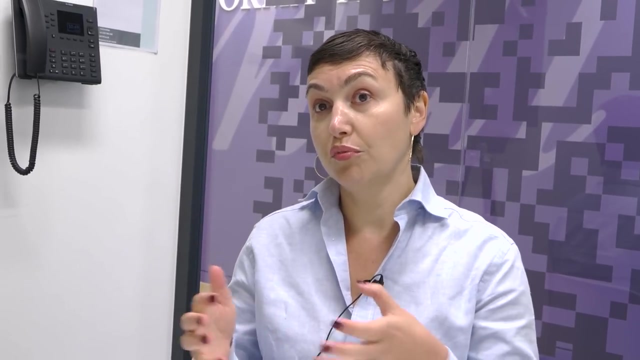 and so the knowledge graph. ultimately, you can- you can imagine it as a, as a database that stores facts about things in the world and relations between them, and and we in in AI and in knowledge graph engineering, we distinguish between the actual data- so bush house, National Theatre- and then abstract data, which is 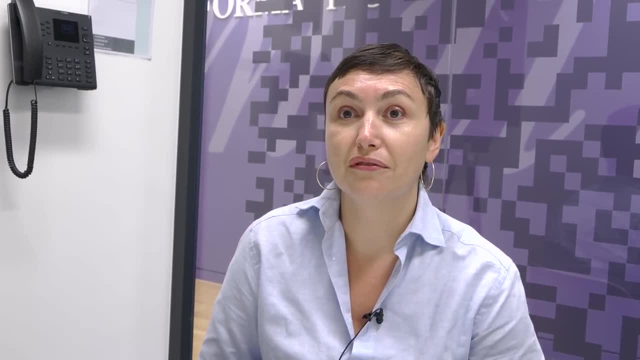 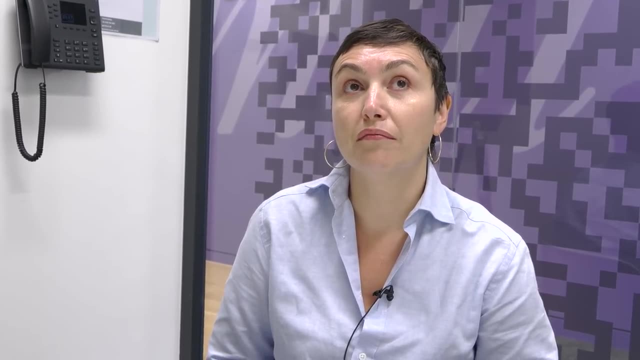 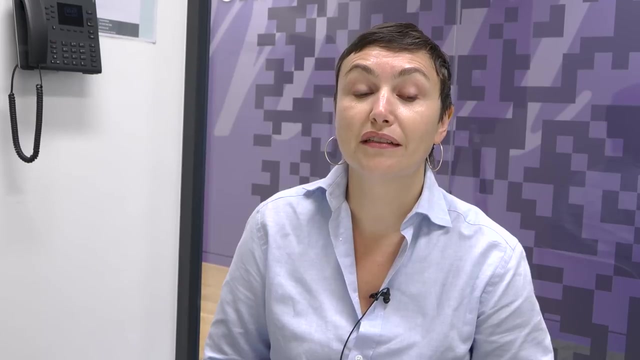 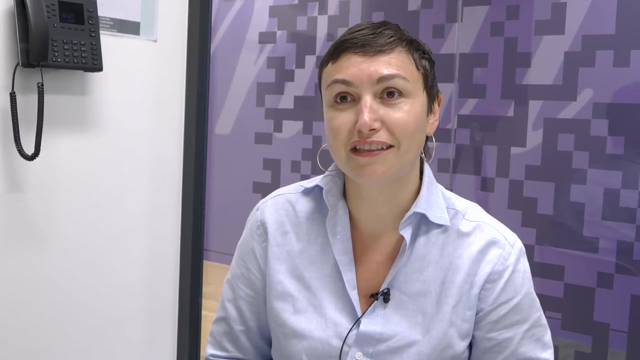 actually, the principles and the technologies have been around for much, much longer, in fact, decades and decades- where AI researchers were building so called knowledge bases, which are very similar types of IT systems that are encoding knowledge, information, data. I don't think we need to go into a big 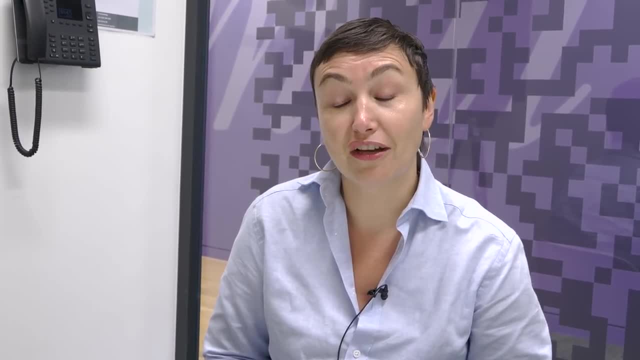 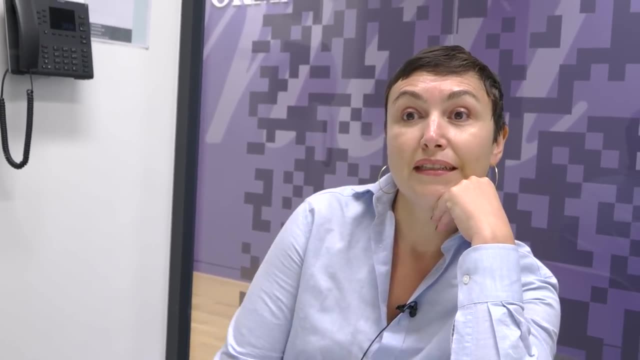 discussion about what these three mean and how they are different from each other. They are In this case, in the example I had, it's about knowledge about London. What connects all these different pieces of data together? So this is the knowledge graph, This is the knowledge graph And the knowledge graph as it is. 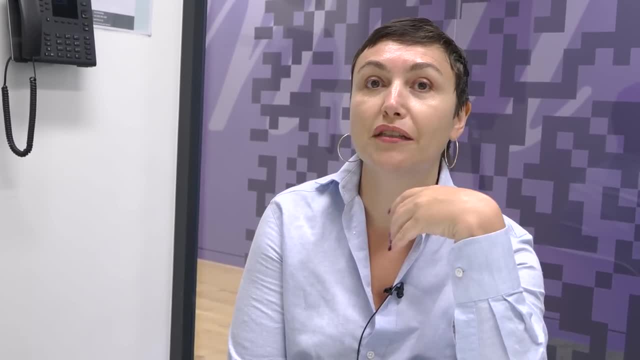 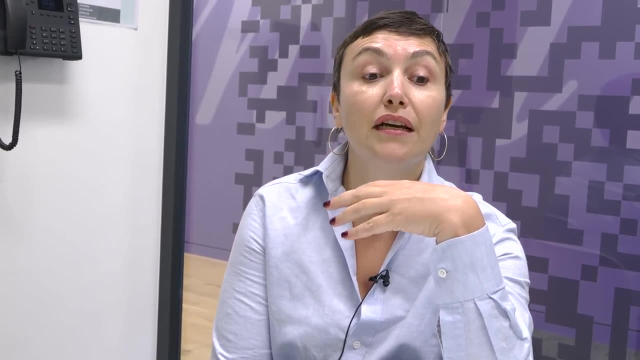 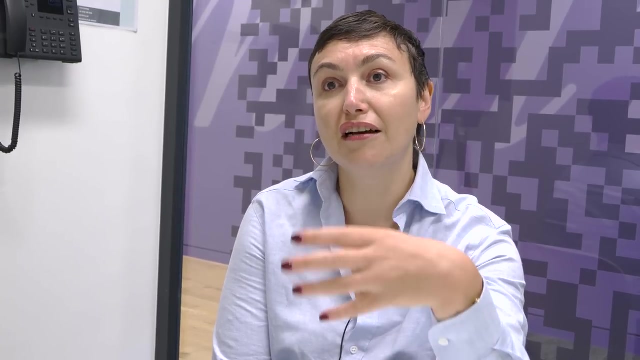 today, not just in the case of Google, but much any large organization that that provides this sort of internet information services, has one. They are huge databases with billions and billions of facts, like this: Bush House is located in London and at this address, right This. 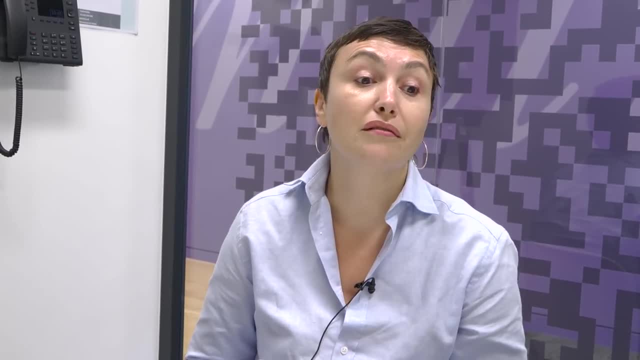 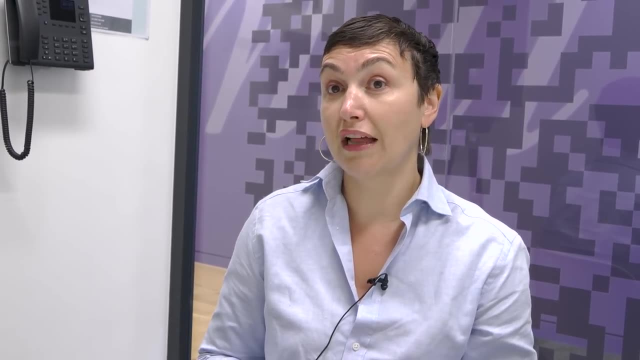 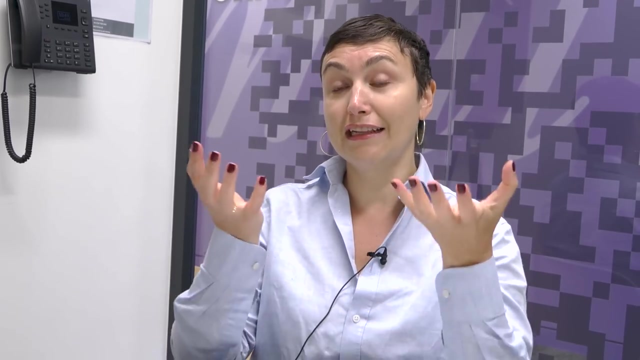 information is extracted from documents, Say on the King's website, somewhere there is information about Bush House and and it's written, probably in text, and Google has the machinery to process all this text and recognize that this string Bush House is probably a building and learn that information, that 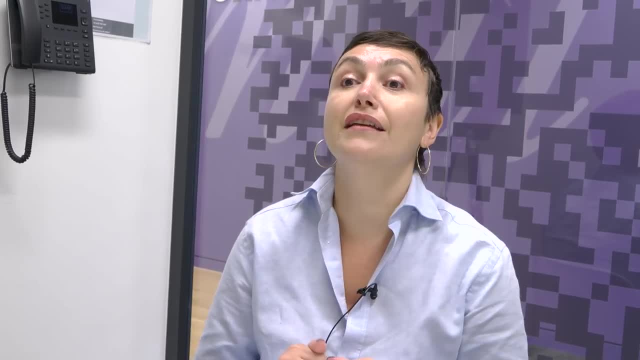 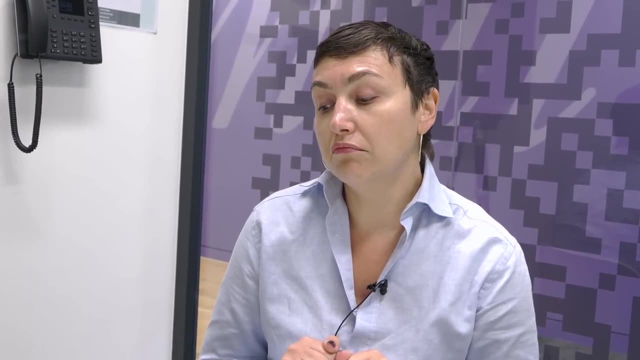 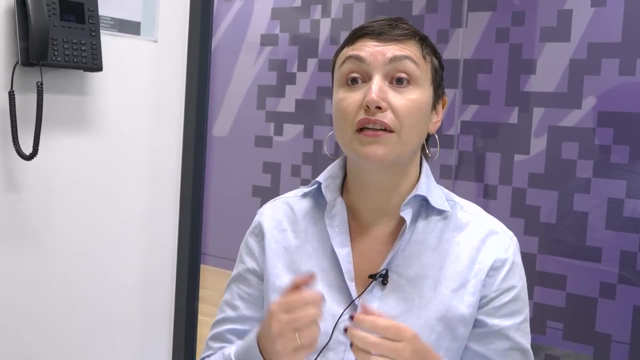 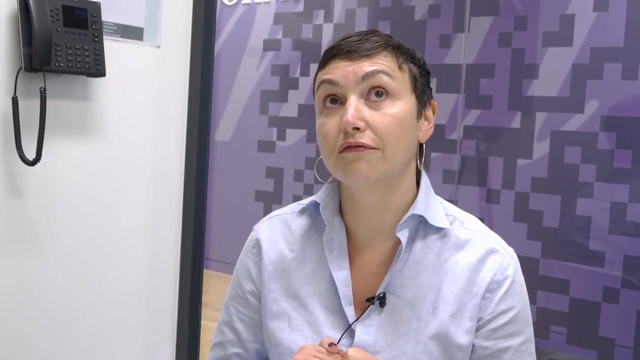 structured information and store that in the knowledge graph. So the knowledge graph, ultimately you can. you can imagine it as a, as a database that stores facts about things in the world and relations between them. And we in AI and in knowledge graph engineering, we distinguish between the actual data. 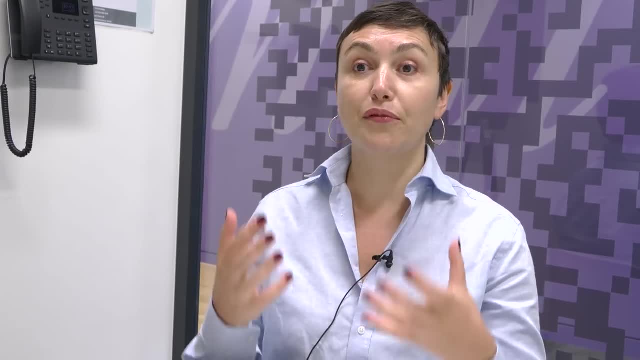 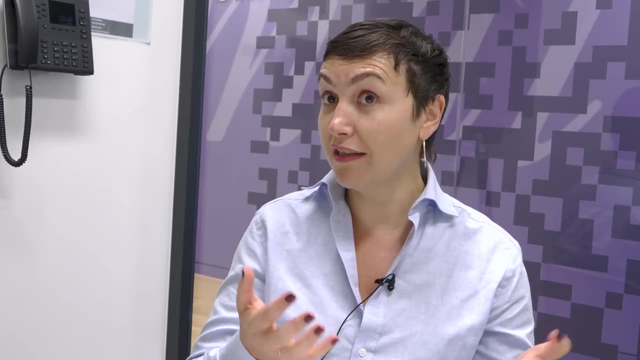 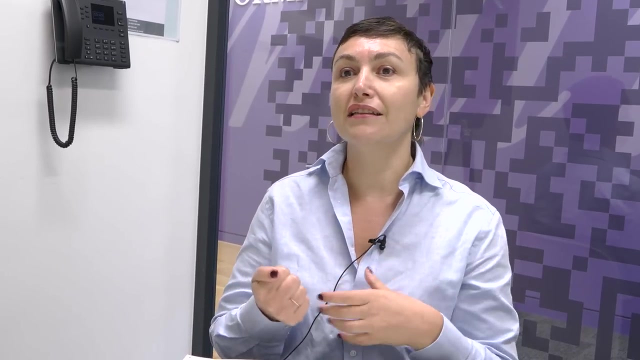 say Bush House, National Theatre, and then abstract data, which is theatres, buildings, universities, So any university, most universities in the world, will have a set of common properties, right, They will teach students, they will be located on a certain campus, They will. 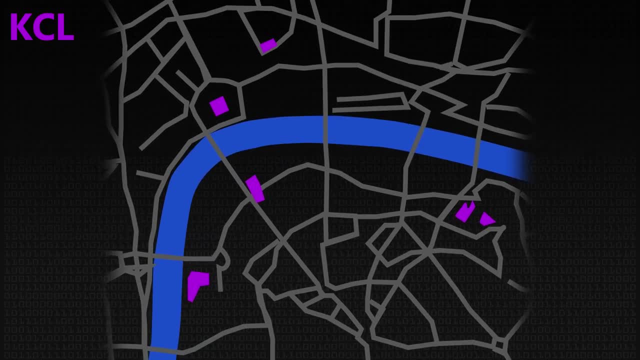 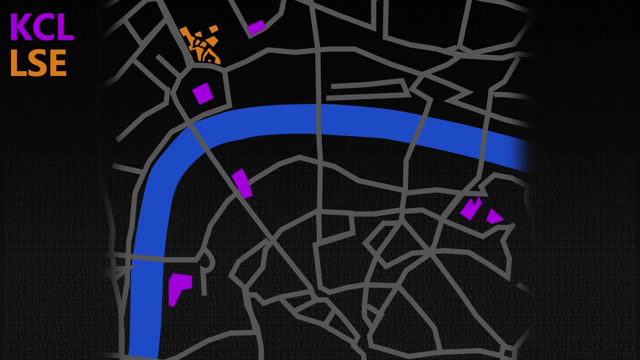 have a certain number of employees. King's College London has three or four actually different campuses. LSE also a university, shares many types of properties, also teaches students, also has employees, but has different campuses, different address. So there is the data about LSE. 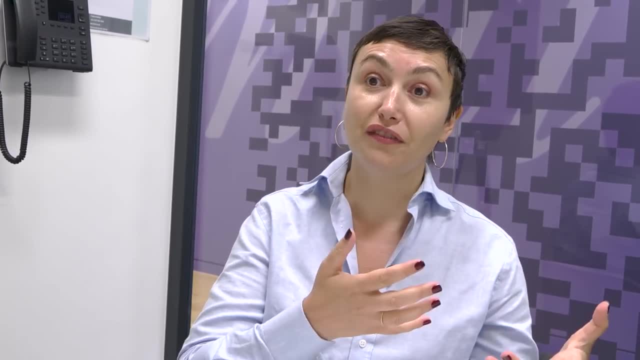 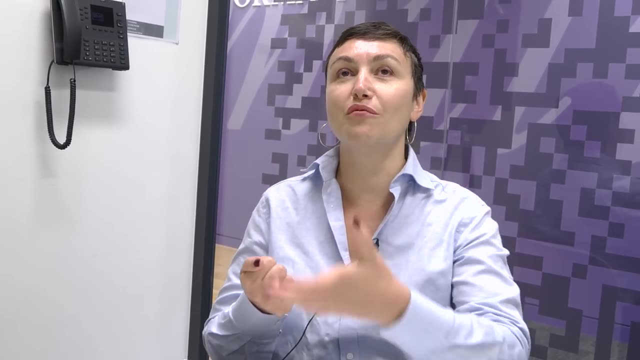 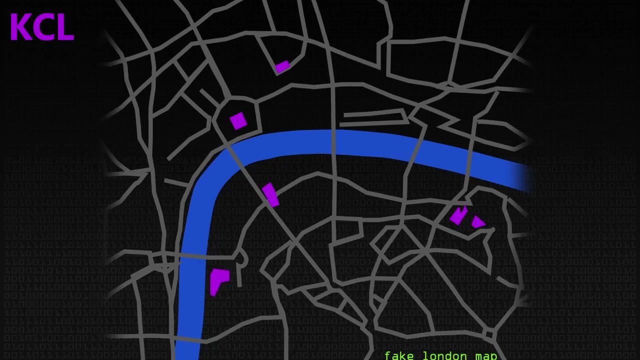 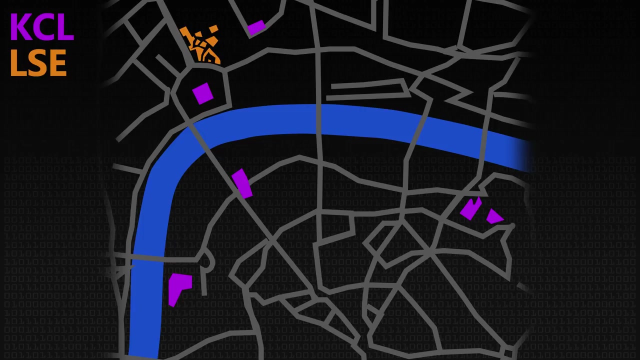 theaters, buildings, universities. so any universe, for most universities in the world, will have a set of common properties. right, they will teach students, they will be located on a certain campus, they will have a certain number of employees. King's College London has three, four actually different campuses. LSE also University shares many types. 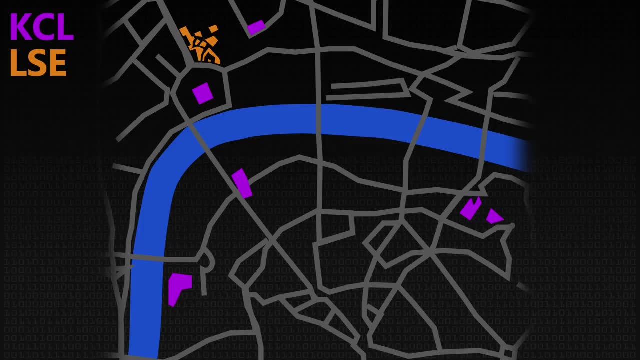 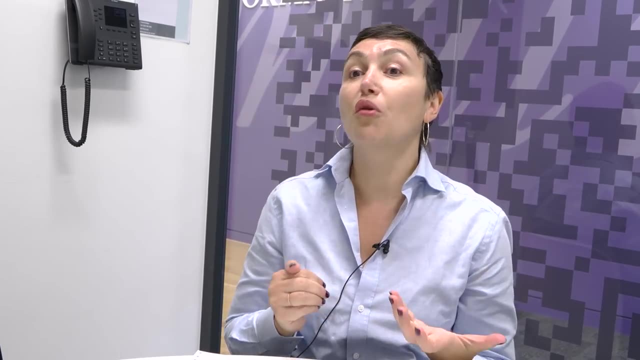 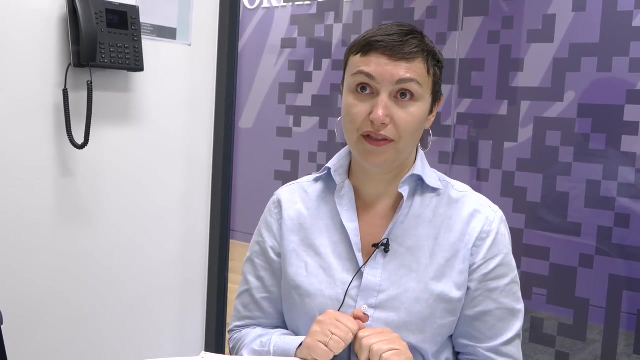 of properties also teaches students, also has employees, but has different campuses, different address. so there is the data about LSE in King's College London and there's all these joint properties that all types of things like LSE, like King's College, have and that helps in web. 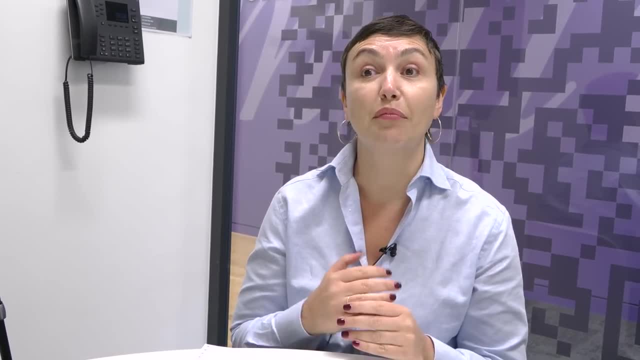 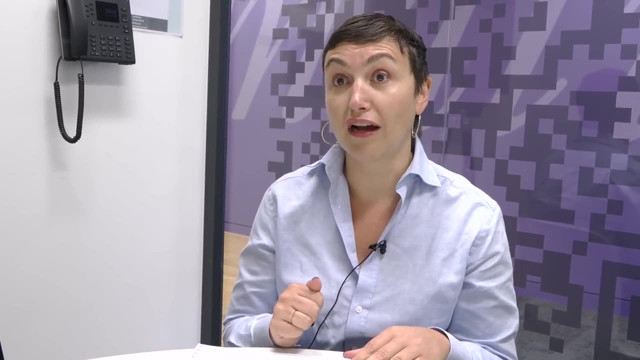 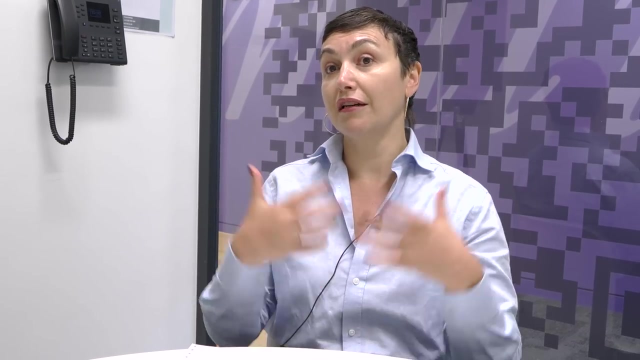 search, but in many other types of AI applications as well. so, in question answering, in recommendations of movies, of products and so on and so forth, because it basically allows that recommender or search engine to provide very specific, very accurate, to the point answers, rather than relying on. 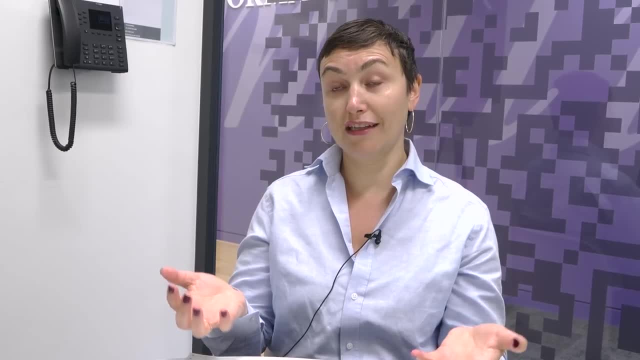 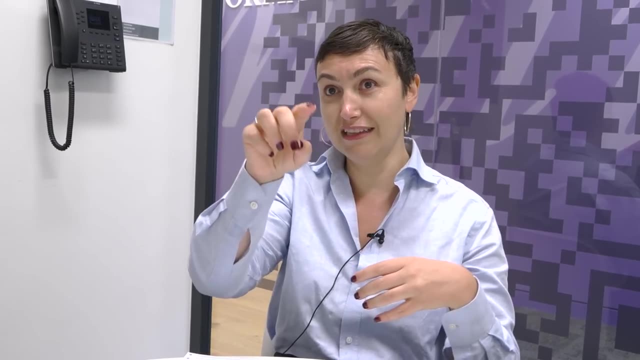 extracting those answers from natural text and you see the difference actually in search, when sometimes you type something and Google says: well, people also asked for this and this, right, and then you have that question and you have that little drop down list and the snippet answer. now some of those answers: 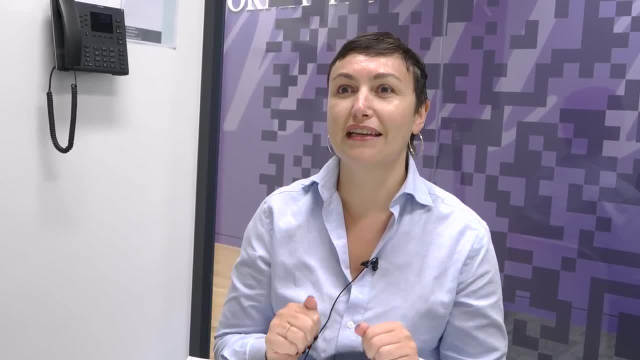 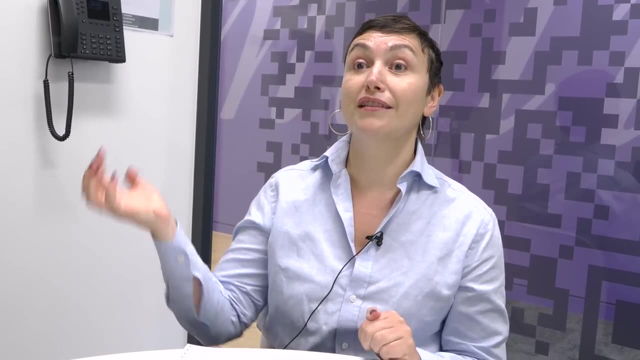 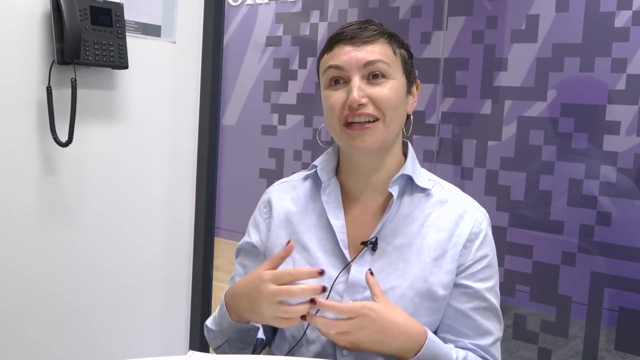 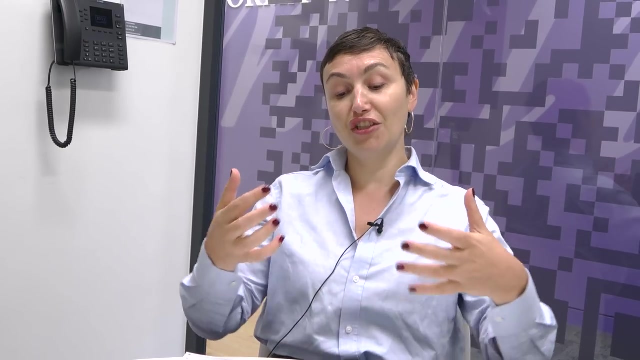 sometimes match what you're looking for, but sometimes they're actually only remotely or not all relevant, and that's the difference your computer has struggles to process and extract very specific types of information from what we call unstructured data- images, text, images, videos- but it has no issue whatsoever, or much less issue to work. 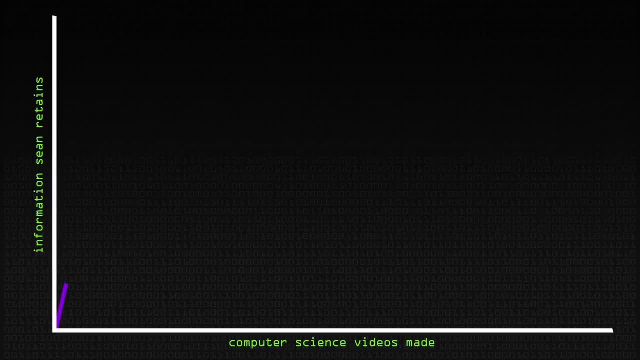 with data that is already structured in a graph, for instance, My simplistic view of graph being a thing you plot on a piece of paper. you know axes Beyond paper you could have many more axes. Is this what we're looking at here? 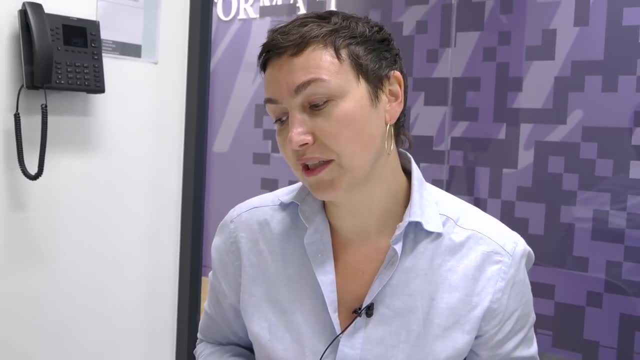 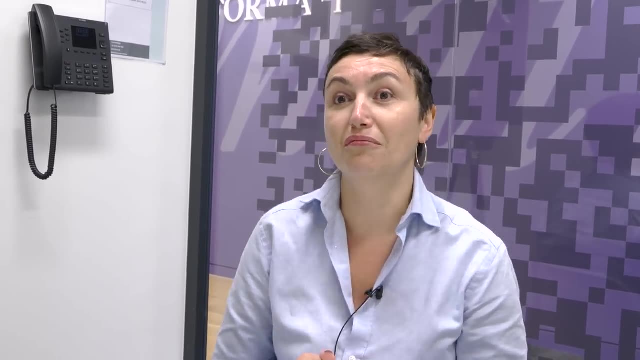 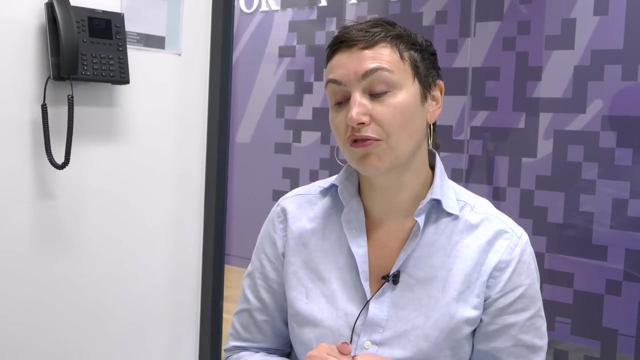 So we're not talking about charts, right? So we're not talking about visually displaying data in a two-, three- or multidimensional visual space. We're talking about a graph in a mathematical sense, So a graph consists of nodes and edges. 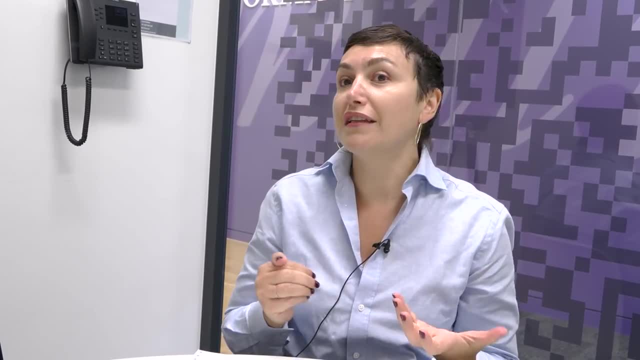 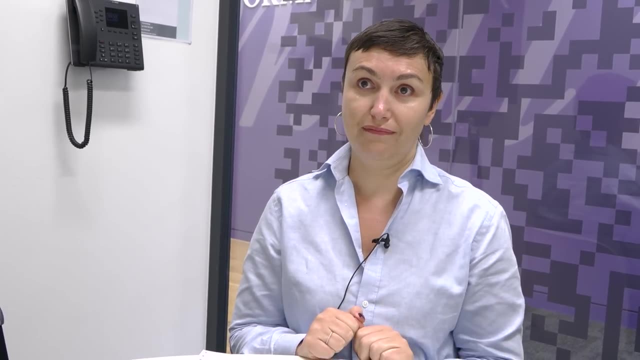 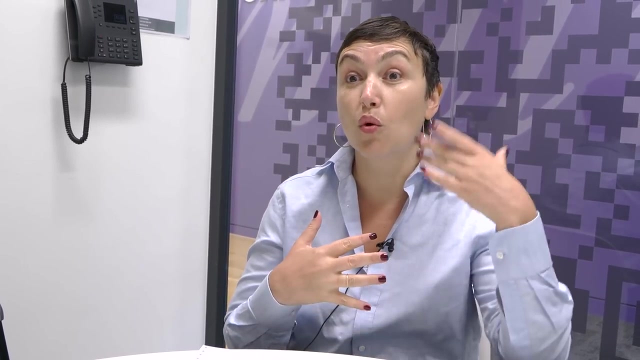 and King's College London and there's all these joint properties that all types of things like LSE, like King's College, have And that helps in web search but in many other types of AI applications as well, So in question answering, in recommendations of movies and products, and so on. 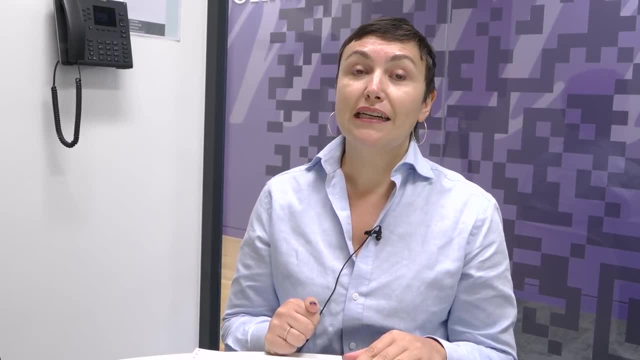 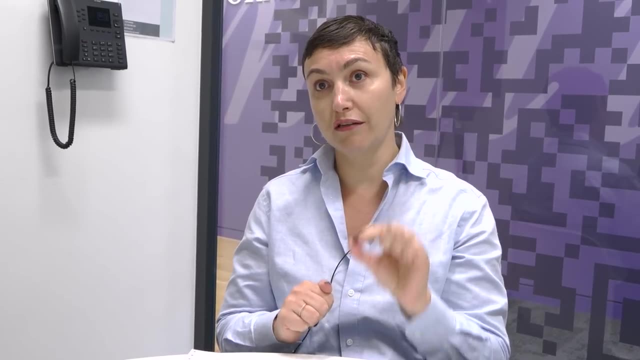 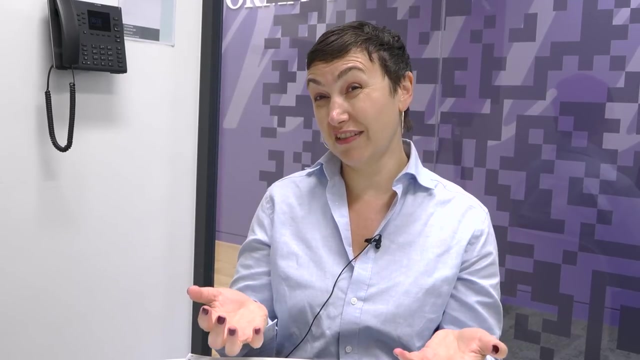 and so forth, because it basically allows that recommender or search engine to provide very specific, very accurate, to the point answers rather than relying on extracting those answers from natural text. And you see the difference actually in search, when sometimes you type something and Google says: well, people also asked for this and this right. 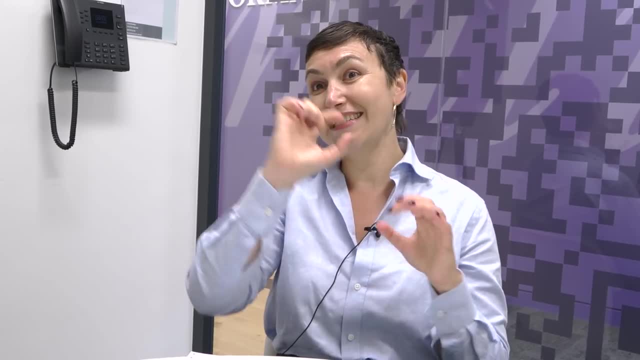 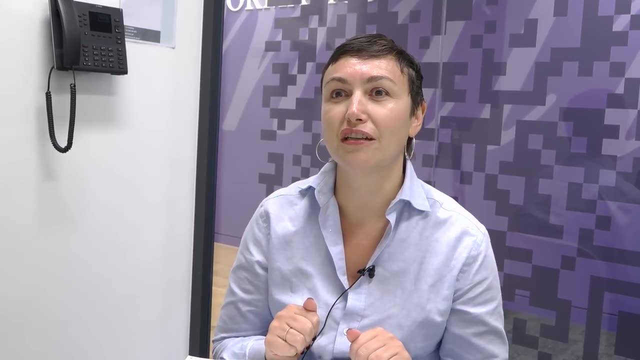 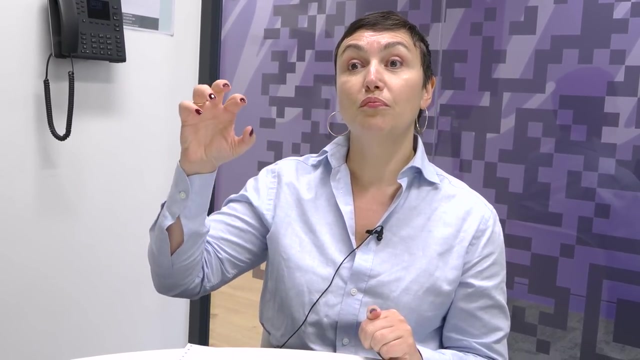 And then you have that question and you have that little drop down list and a snippet answer. Now, some of those answers sometimes match what you're looking for, but sometimes they're actually only remotely or not all relevant, And that's the difference A computer has struggles to process. 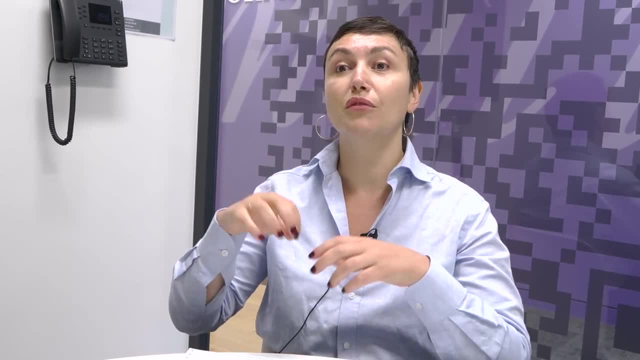 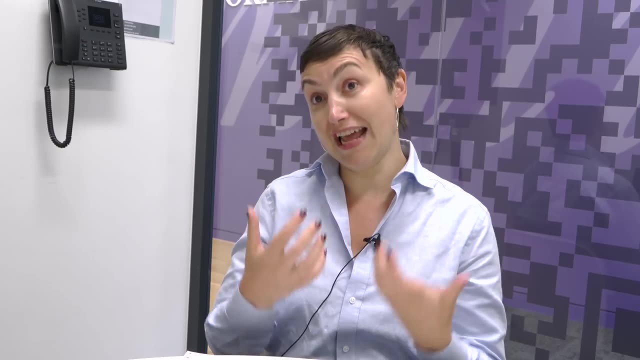 and extract answers, And so it's a little bit of a challenge to be able to do that. A computer can extract very specific types of information from what we call unstructured data, which is text, images, videos, but it has no issue whatsoever, or much less issue, to work with data. 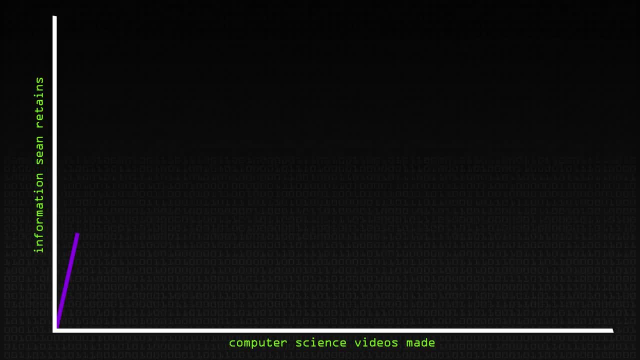 that is already structured in a graph, for instance, My simplistic view of graph being a thing you plot on a piece of paper. you know axes beyond paper, you could have many more axes. Is this what we're looking at here? So we're not talking about charts, right? So we're not talking about. 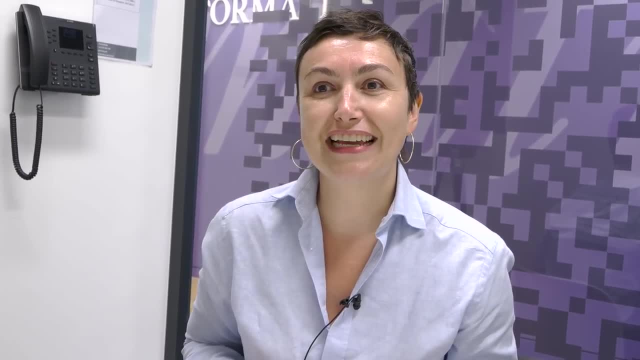 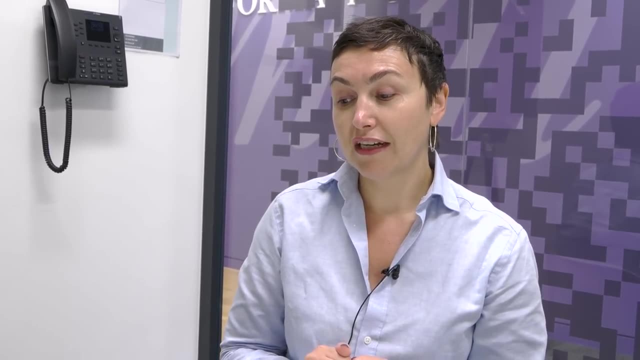 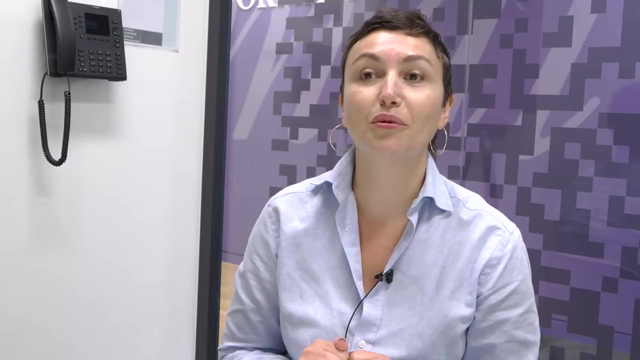 um visually displaying data in a two, three or multidimensional visual space. We're talking about a graph in a mathematical sense. So a graph consists of nodes and edges. Um, we know graphs from computer networks, right? So you have um computers which are the nodes and then the 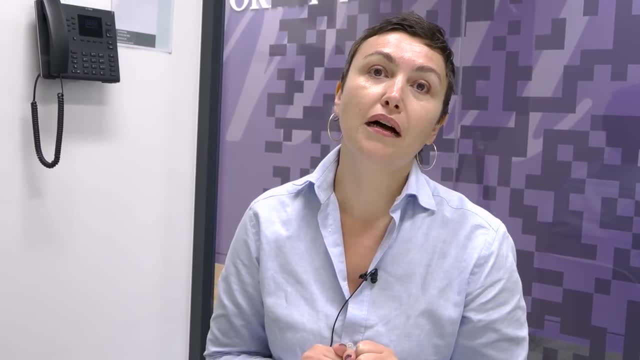 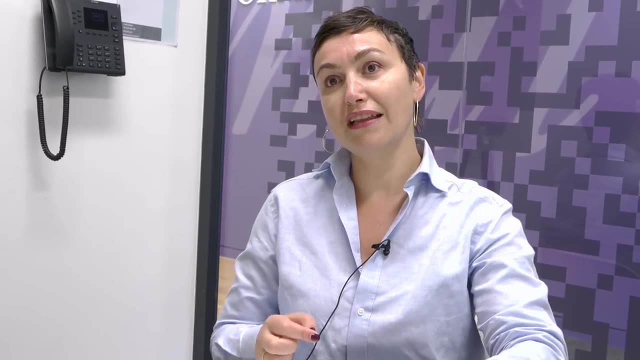 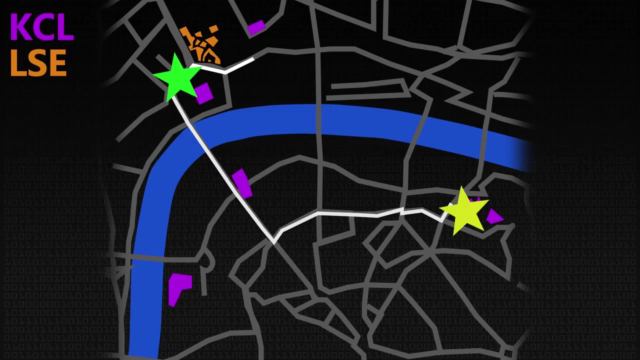 communication links between them. We know graphs from um, geospatial information systems maps- right, So you have points on a map and then you have roots. You need all sorts of algorithms to compute edges, for instance in the case of maps, If you want to go from A to B. 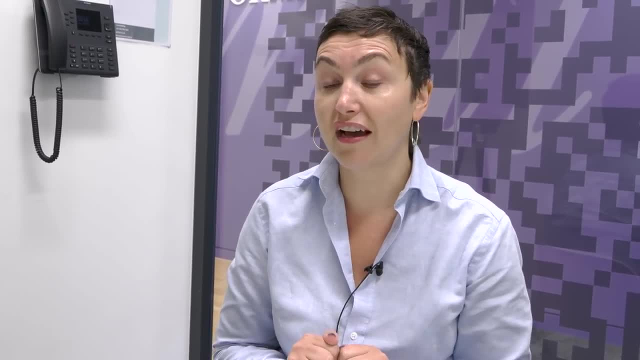 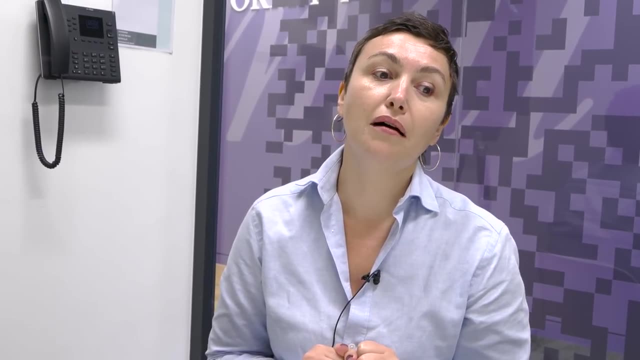 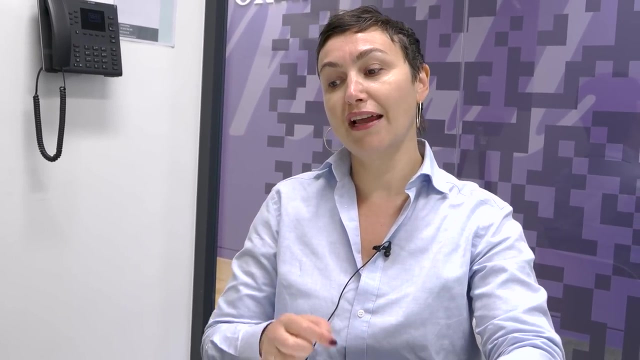 We know graphs from computer networks- right, So you have computers which are the nodes and then the communication links between them. We know graphs from geospatial information systems, maps- right. So you have points on a map and then you have roots. 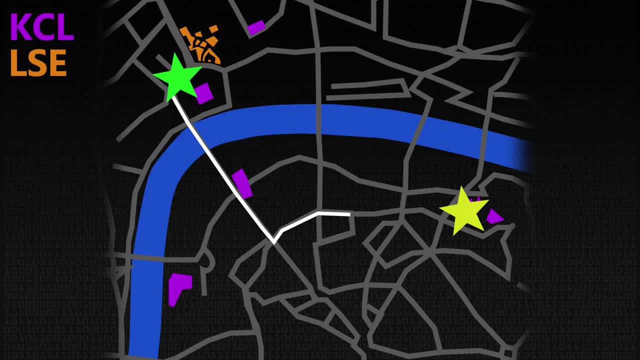 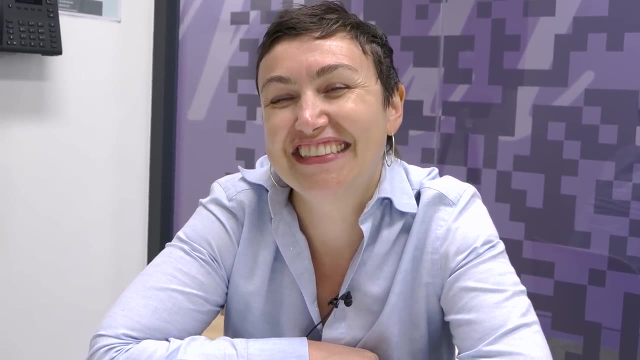 You need all sorts of algorithms to compute edges. for instance, in the case of maps, If you want to go from A to B, you can do that by passing multiple intermediary nodes. So when you say an edge, I mean we kind of had the example of a map and that being a. 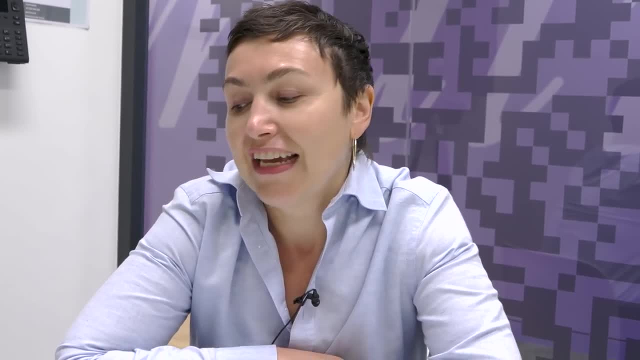 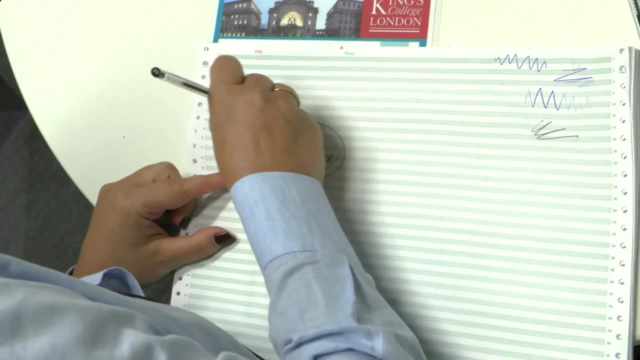 root in the map. Yes, How do you define an edge? Well, it's, it's any type of relation, right? So for Bush House it could be: has address. So let's just say that we represent the nodes in these ovals and then we represent the. 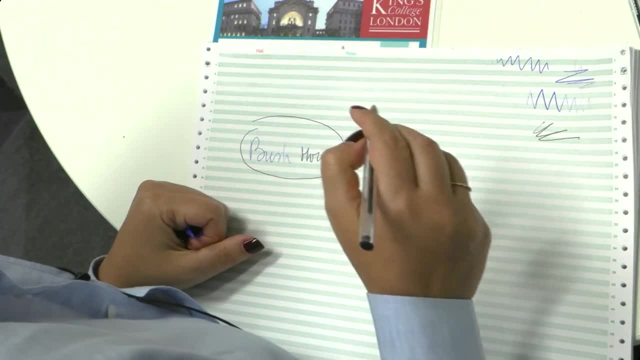 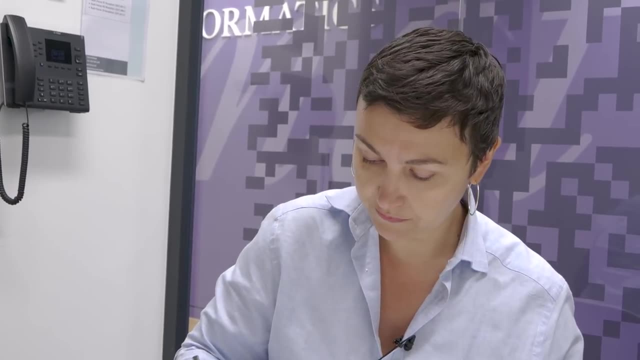 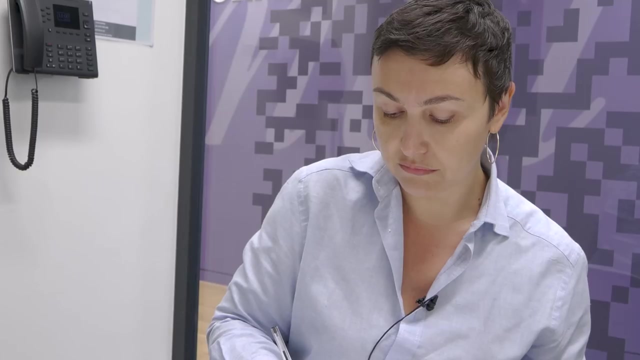 edges as lines between these nodes. So we're talking about Bush House and we're talking about King's College, London, right And then? so what's the relationship between Bush House and KCL, Campus of, or something? Yeah, Campus of, or we could call it building of KCL? 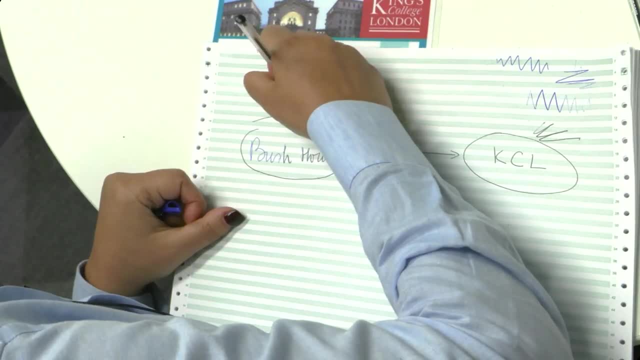 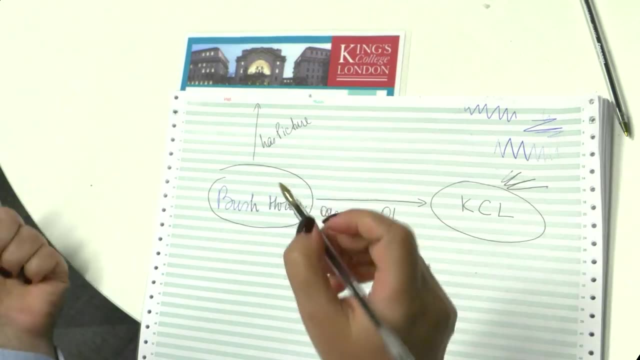 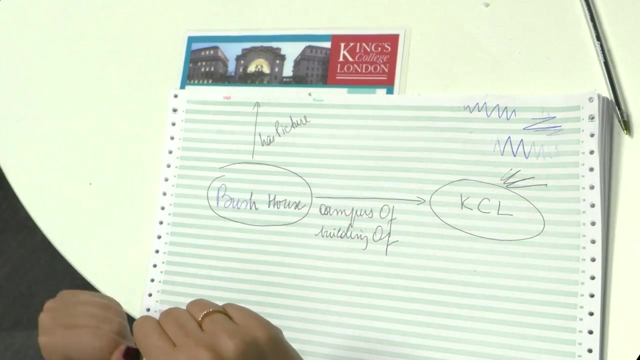 We can have another relationship that says: Bush House has picture, And here's my picture of Bush House And it could be an actual image. All these lines can have different meanings So I can have the has picture edge from Bush House, from KCL, you could have something. 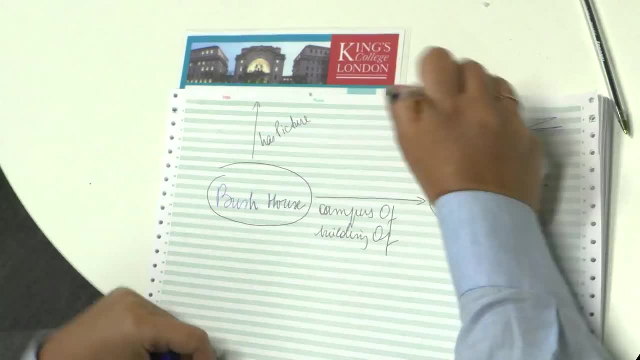 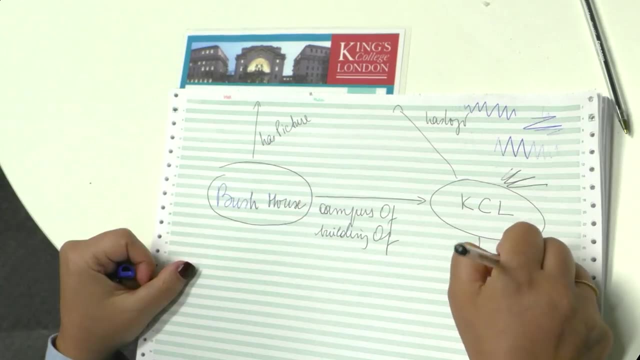 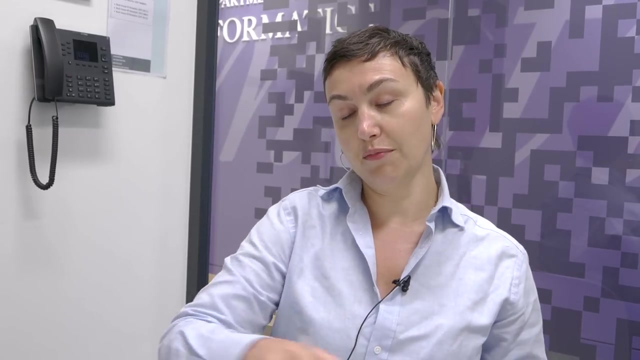 like has logo. I've pointed out, Yeah, And it points to another image. that is the logo. You could also have some sort of has picture with some picture of KCL, who knows, And there's an image file here So you can have different types of edges. 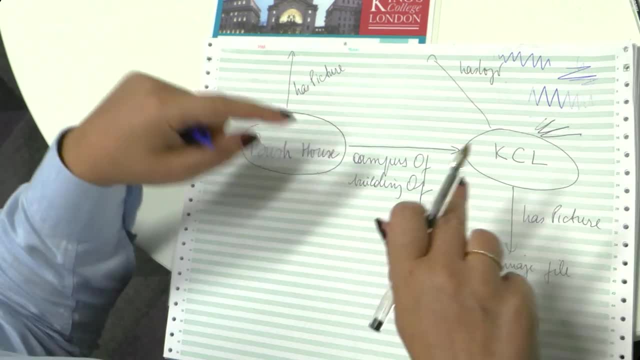 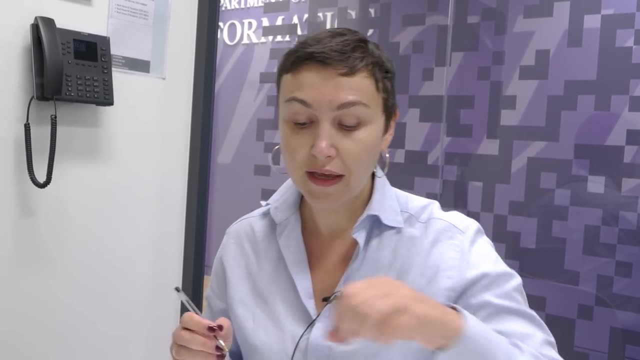 This type of has picture edge and this one here are the same. So if you want to have all pictures of things, you can query, just like you would query with SQL in a database. You can have any type of edge you want. You label it. 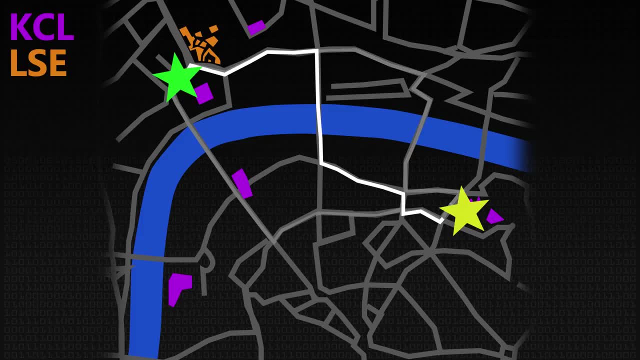 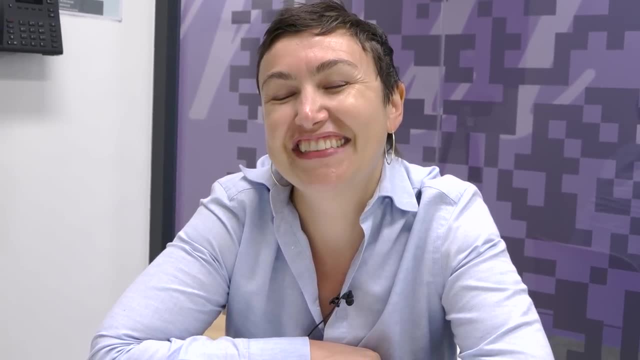 you, um, can do that bypassing multiple intermediary nodes. So when you say an edge, I mean we- we kind of had the example of a map and that being a route in the map. Yes, Well, what, how do you define an edge? 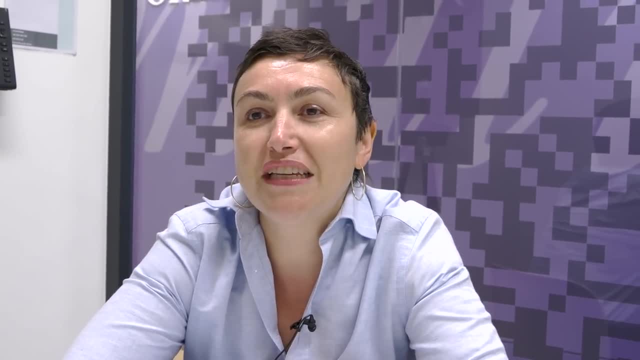 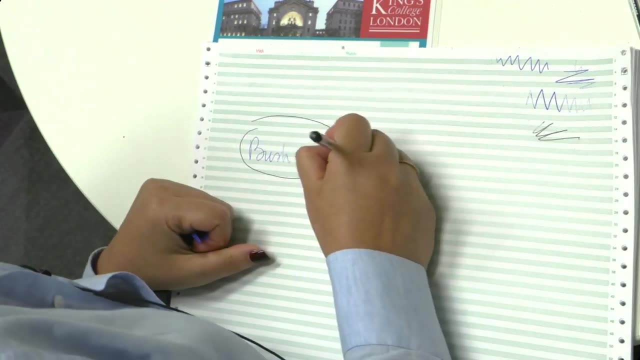 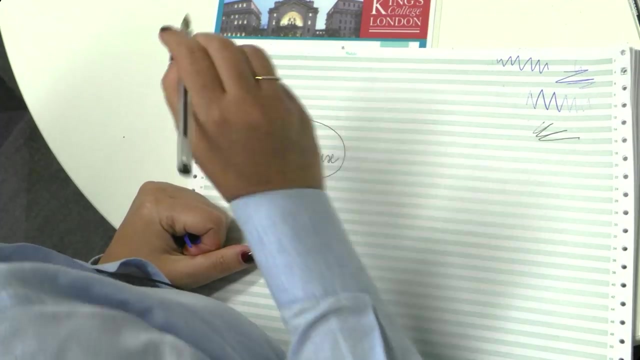 It's any type of relation right? So for Bush House it could be. has address. So let's just say that we represent the nodes in these ovals and then we represent the edges, as uh lines between these nodes. So we're talking about Bush. 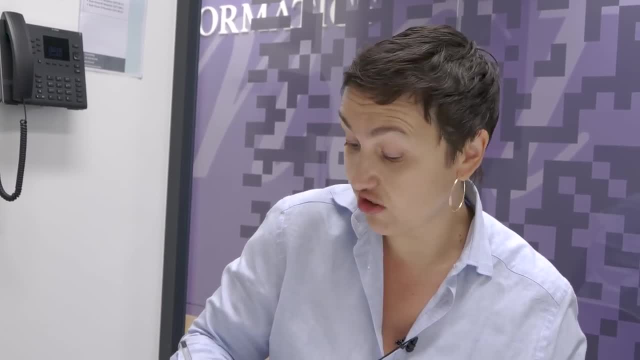 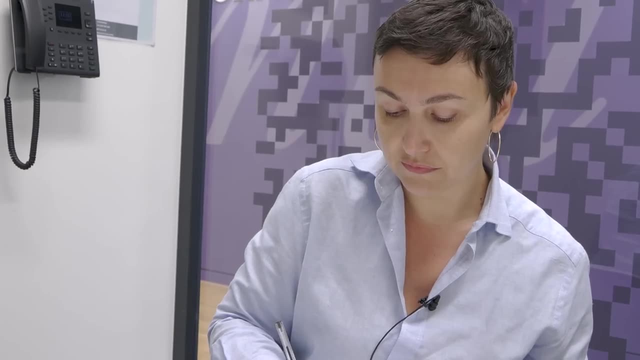 House, and we're talking about King's College, London, right, And then? so what's the relationship between Bush House and KCL Campus of, or something? Yeah, Campus of, or we could call it campus of, Campus of, or we could call it campus of. 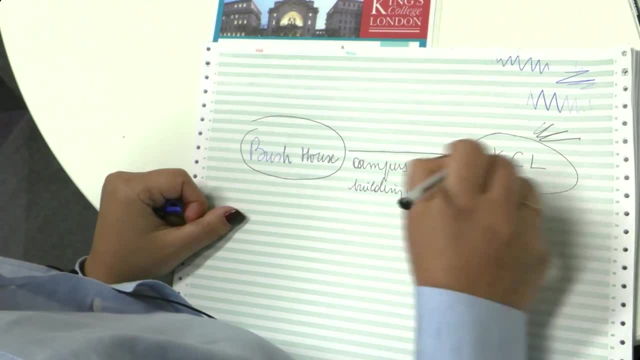 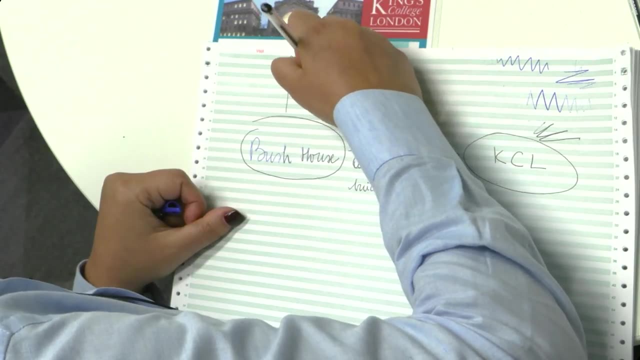 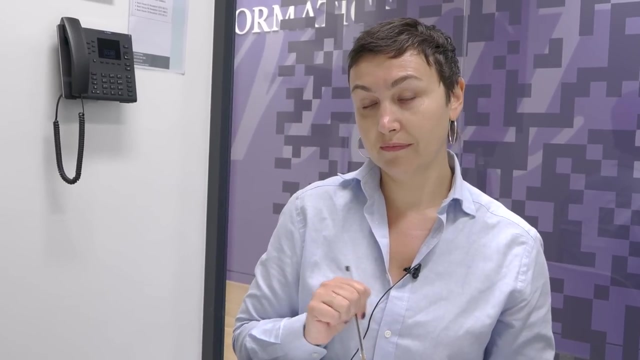 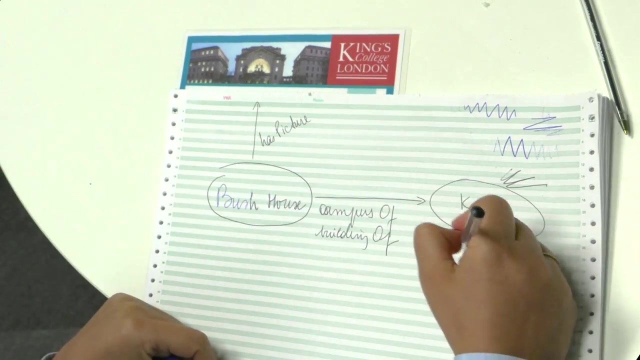 Campus of, or we could call it building of KCL. We can have another relationship that says: Bush House has picture And here's my picture of Bush House And it could be an actual image. All these lines can have different meanings So I can have the has picture edge from Bush House, from KCL. You. 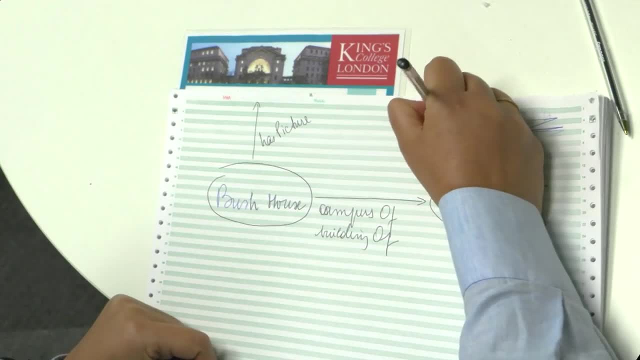 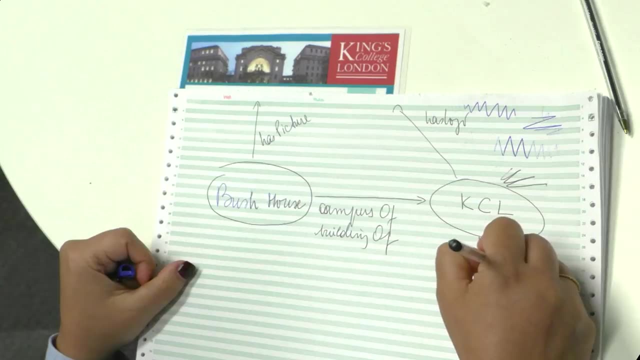 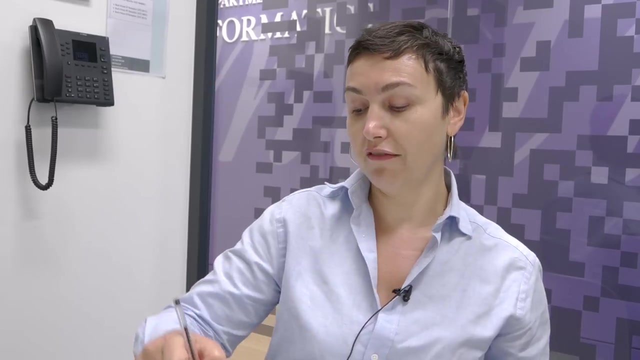 could have something like: uh, has logo. This kind of image points to another image That is the logo. Um, you could also have some sort of has picture with some picture of KCL, who knows, and there is an image file here So you can have. 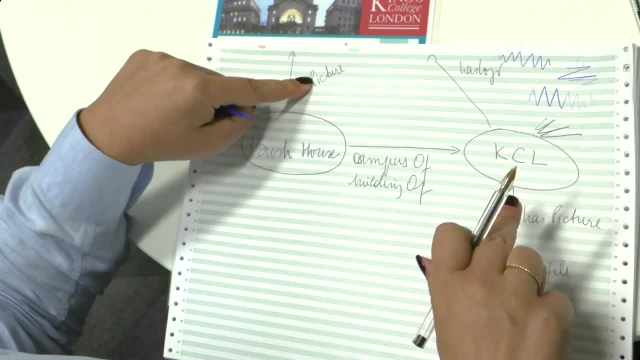 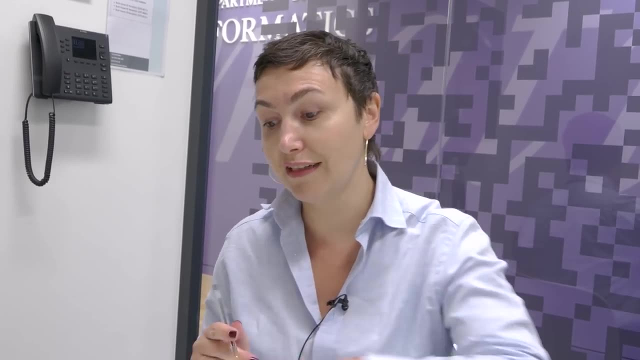 different types of edges. This type of has picture edge and this one here are the same. So if you want to have all pictures of things, you can query, just like you would query with sweet sequel in a database. Um, you can have any type of edge you want. 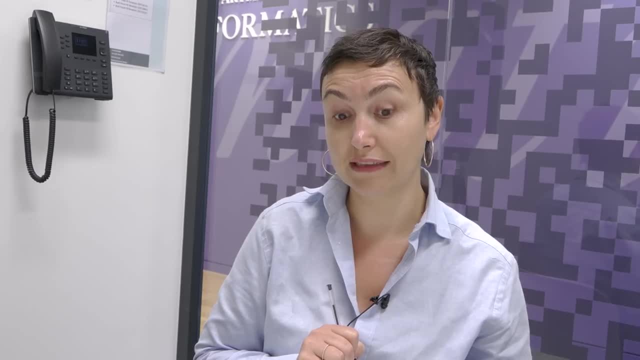 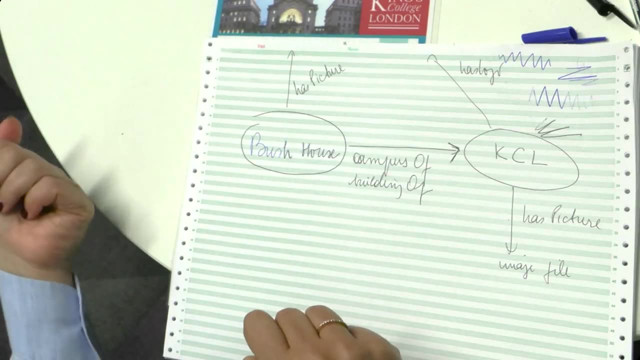 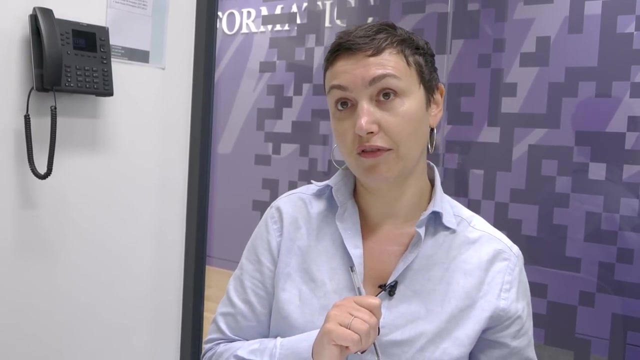 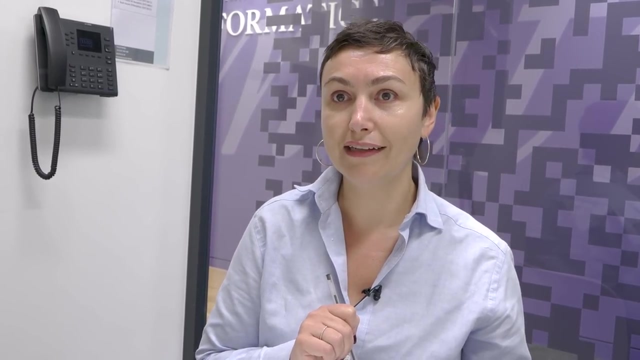 mine have arrows. that's mostly just for my understanding, because I want to say that the image is something that belongs to the house and on the other way around, sometimes you have edges that could have arrows on both ends. so if you think about Elena has sibling, Alex, my brother, so the edge has sibling is what. 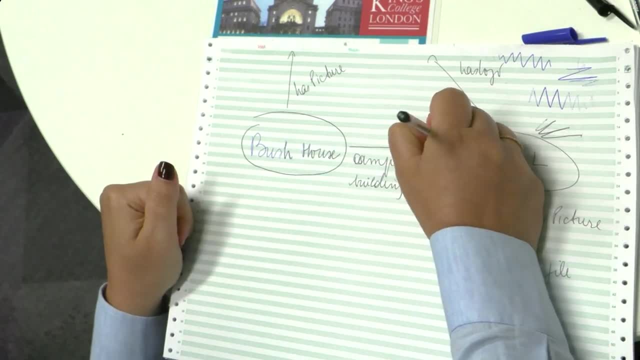 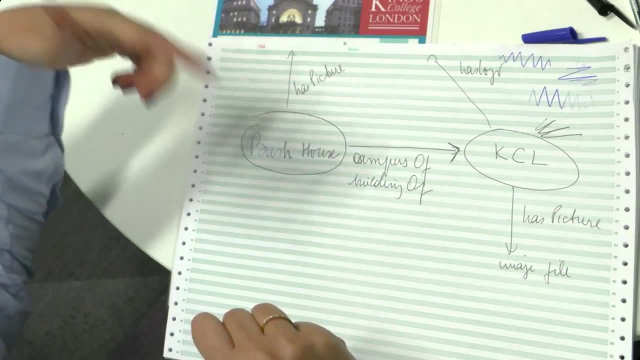 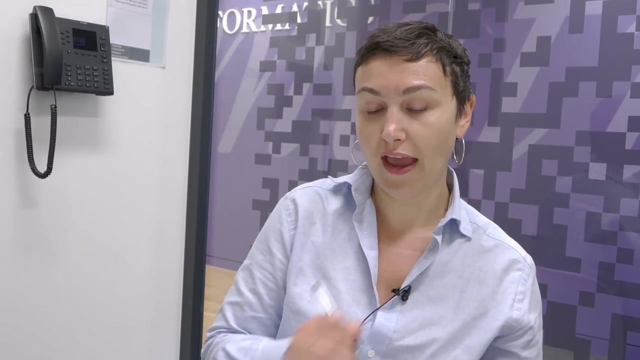 So you give it a name. Mine have arrows. That's mostly just for my understanding, because I want to say that the image is something that belongs to Bush House and not the other way around. Sometimes you have edges that could have arrows on both ends. 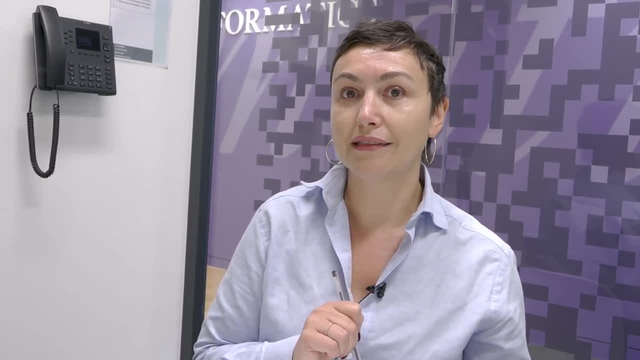 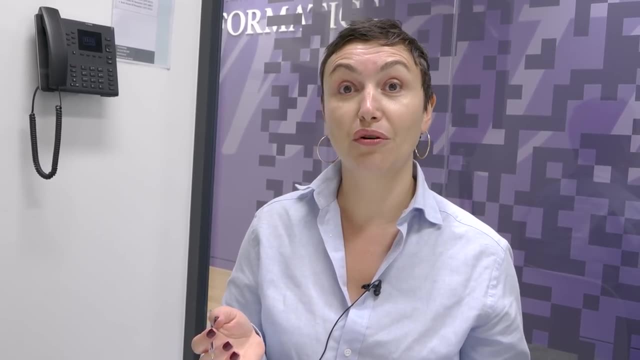 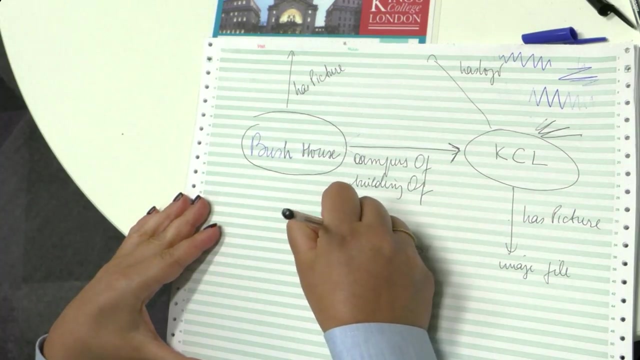 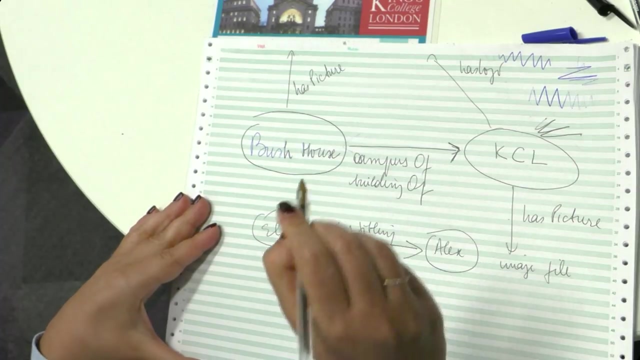 So if you think about Elena has sibling Alex, my brother, So the edge has sibling. Edge has sibling is what we call symmetrical, So if I'm his sister then he's my brother. Say the moment when I define the edge has sibling from the node Elena to the node Alex. 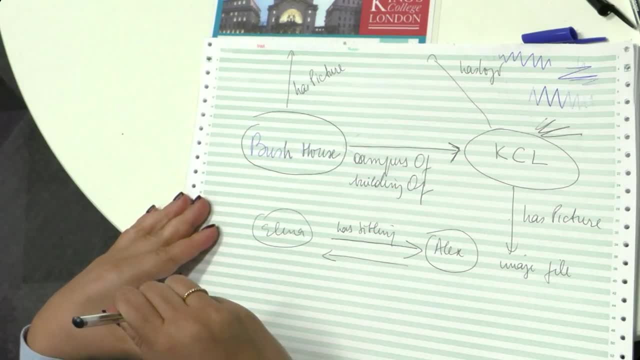 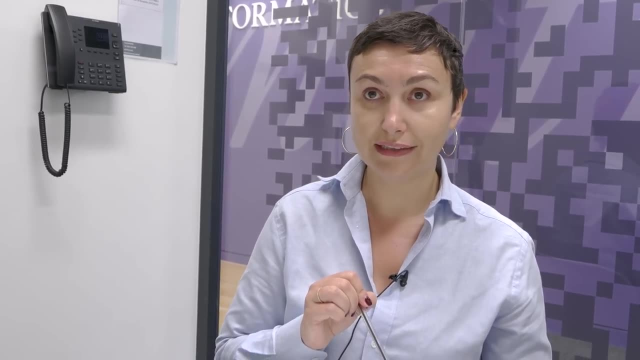 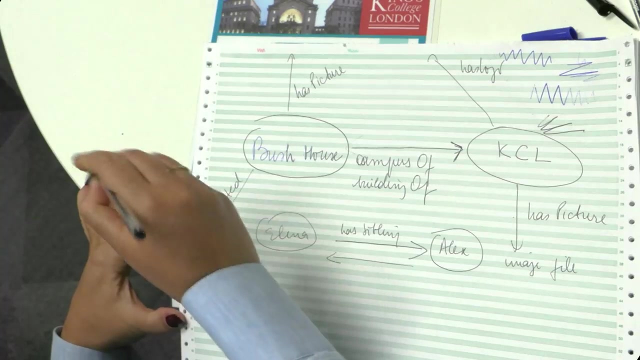 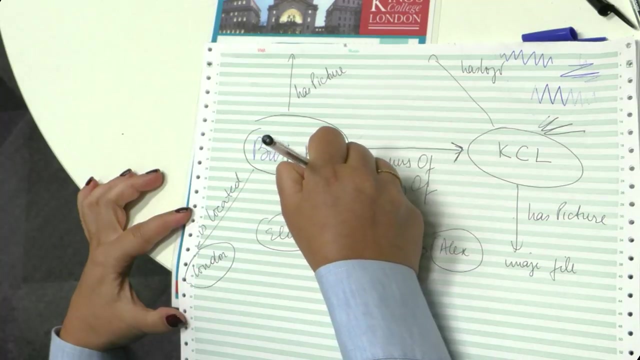 the computer. I can actually tell the computer. by the way, there is also the opposite edge. If I have an edge or a relationship like is located in: So Bush House is located in, So Bush House is located in. You see how the graph actually starts to take shape in London and Elena works at Bush House. 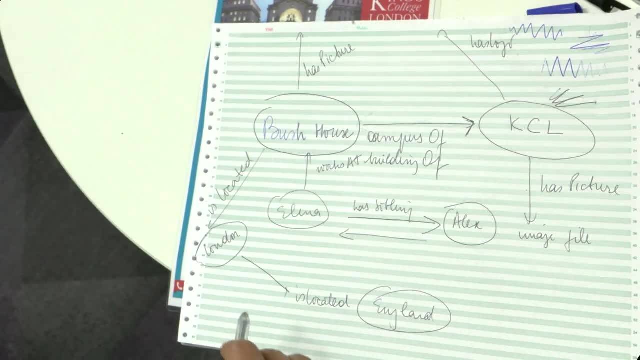 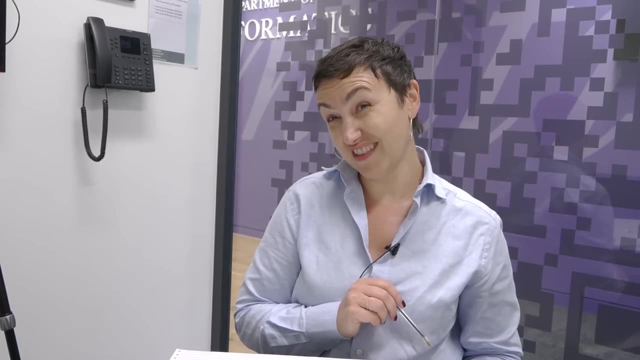 and London is located in England. You can tell the computer well, is located in is a type of edge. that is what we call in math transitive. So if I know that Bush House is located in London, I know London is located in England. 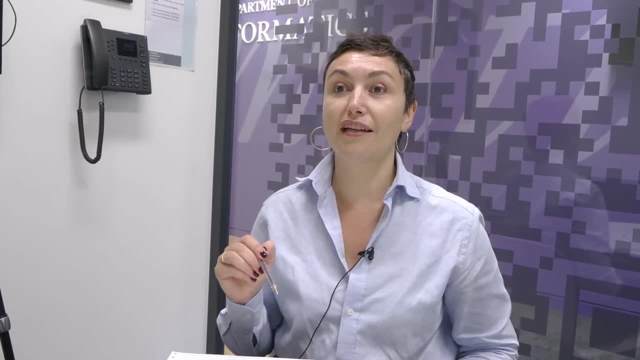 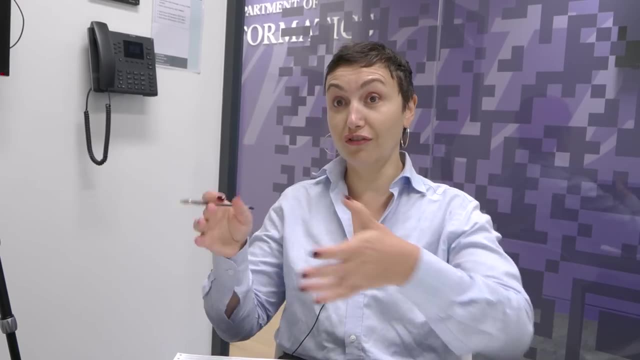 and I know that Bush House is located in England, So you don't actually have to look for that sort of question. if someone ever would ask, is Bush House located in England? You don't actually need to look for the data specifically. you can what you call infer. 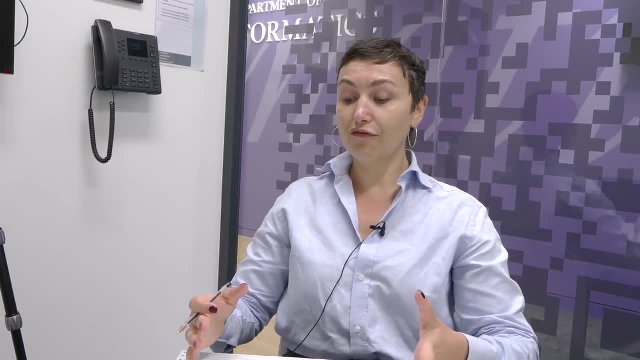 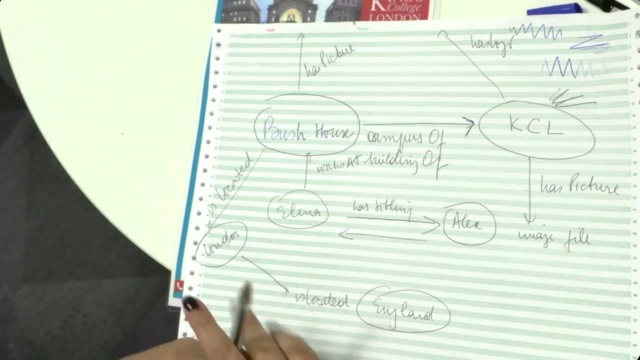 it. So you can. from all this information that I have written down, you can now infer additional knowledge. This is a bit like an ontology. Yes, it is an ontology. Well, it is based on an ontology, to be more specific. So it's based on an ontology, to be more specific. 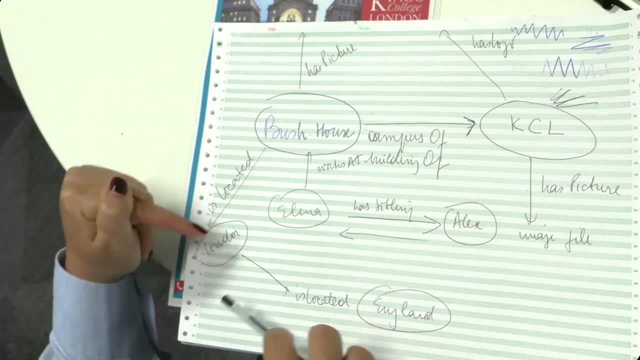 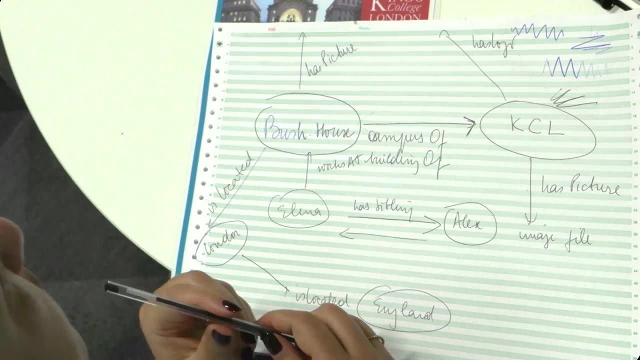 Okay, So it's based on an ontology. to be more specific, The ontology will be something about cities and about buildings, and cities and buildings belonging to institutions and people working in certain buildings. Is there an easy sort of freeway? people could play with this or try this. 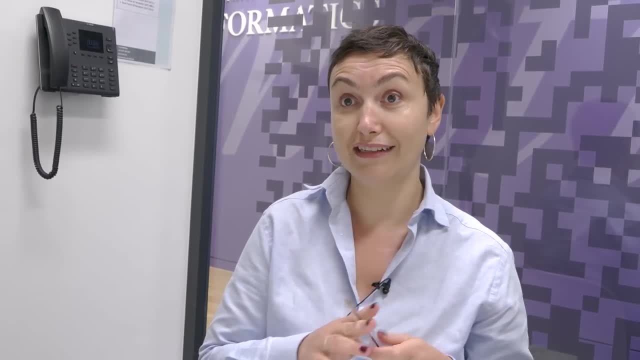 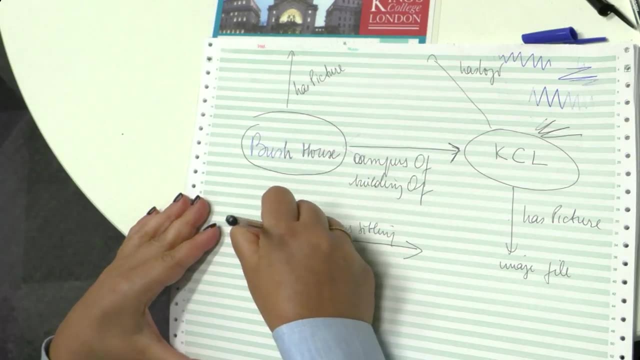 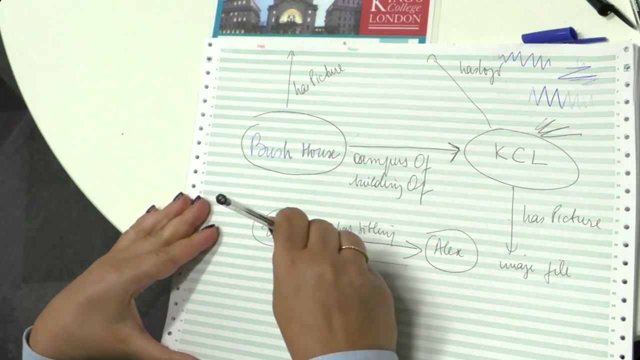 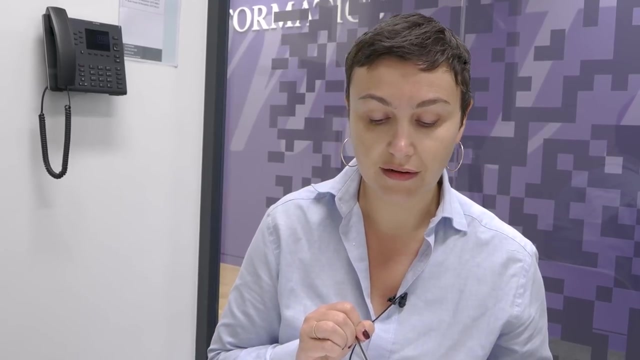 we call symmetrical. so if I'm his sister, then here's my brother. say, the moment when I define the edge has sibling from the note Elena to the note Alex, the computer. I can actually tell the computer. by the way, there is also the opposite edge. if I have an edge or a relationship like is located in the 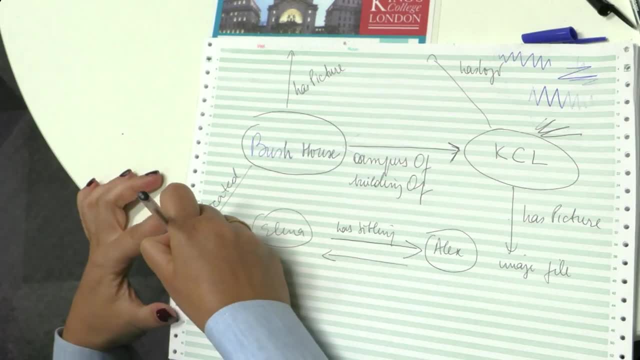 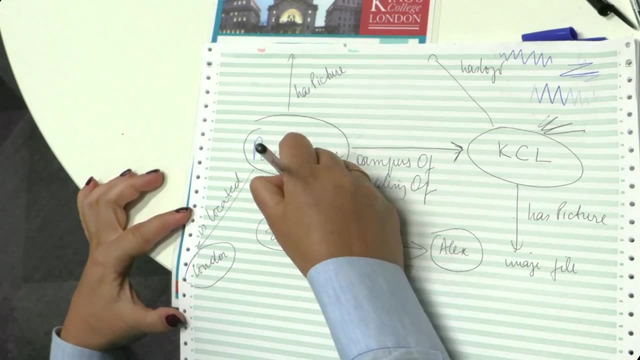 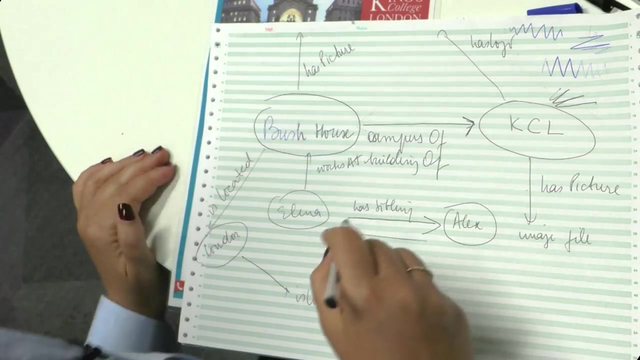 bush house is located in London. you see how. you see how the edge is located in. the bush house is located in London. you see the graph actually starts to take shape in London and Elena works at bush house and London is located in England. you can tell the computer, well, is located in is. 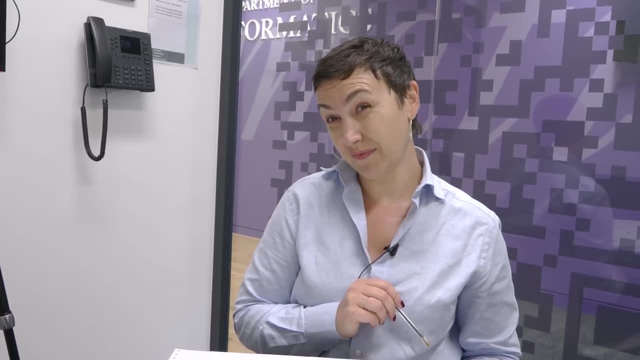 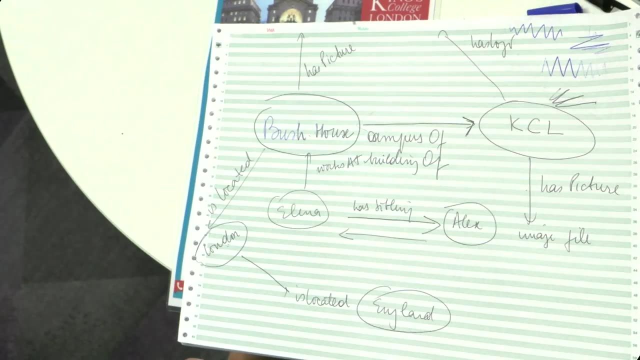 a type of edge. that is what we call in mass transitive. so if I know that Bush house is located in London, I know London is located in England and I know that Bush I was located in England and I know that Bush house is located in England. 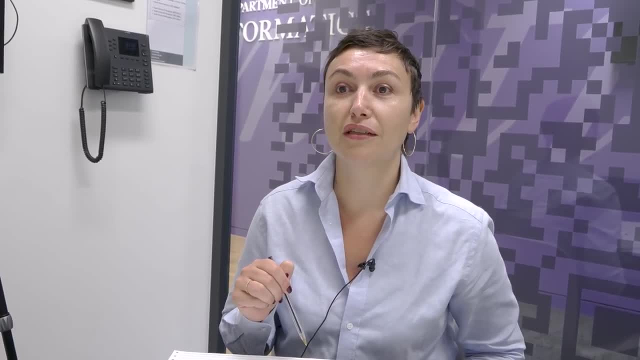 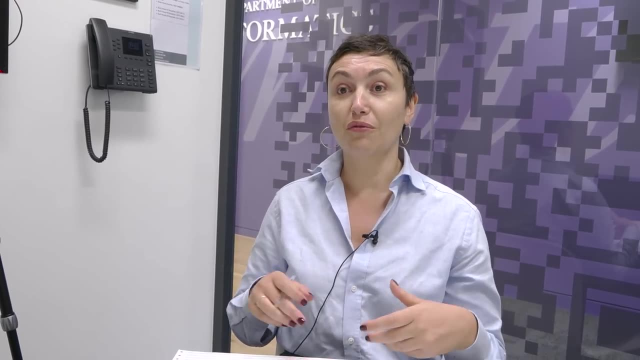 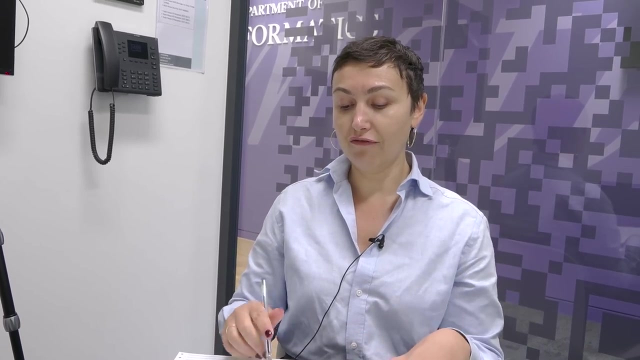 so you don't actually have to look for that sort of question. if someone ever would ask, is Bush house located in England? you don't actually need to look for the data specifically. you can what you call infer it. so you can. from all this information that I have written down, you can now infer additional. 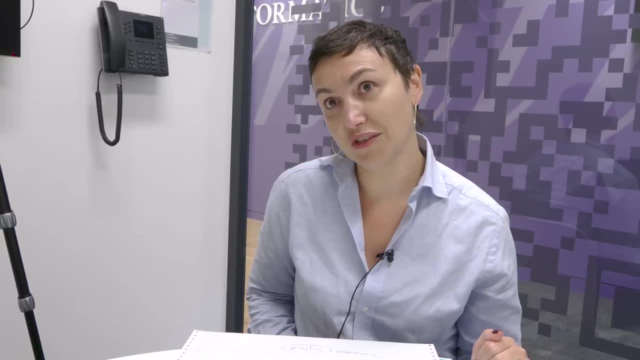 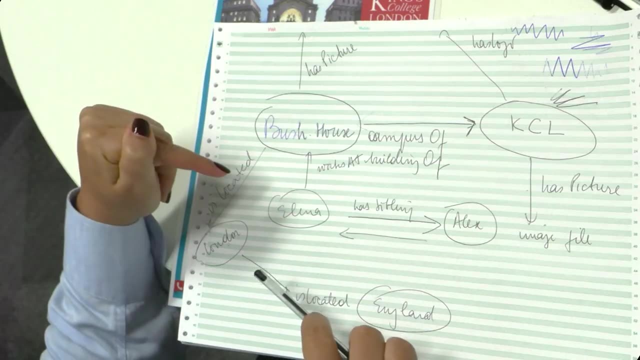 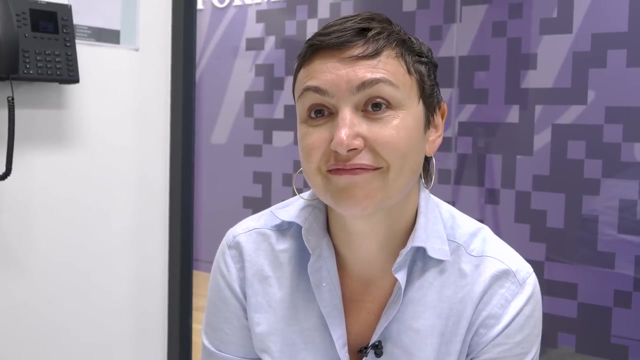 knowledge. this is a bit like an ontology. yes, it is an ontology. well, he's based on an ontology. to be more specific, the ontology will be something about cities and about buildings in cities and buildings belonging to institutions and people working in certain buildings. is there an easy sort of freeway? people could play with this or try this. is there something? 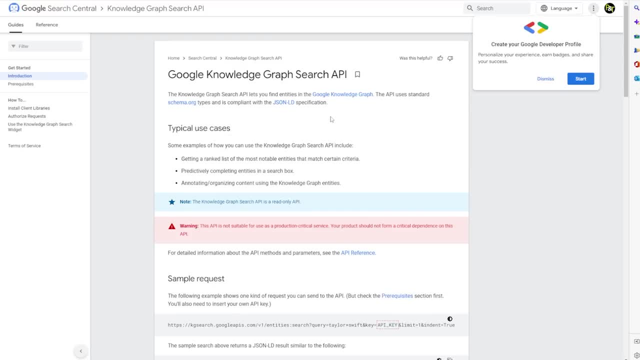 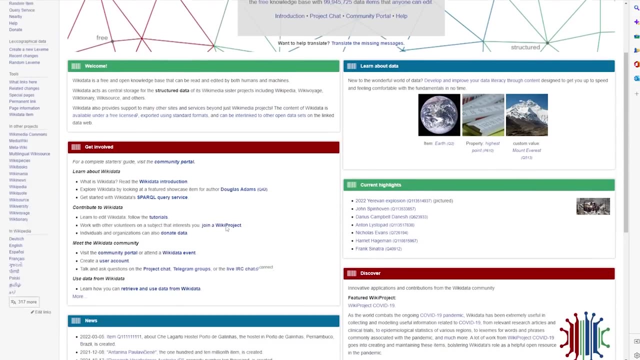 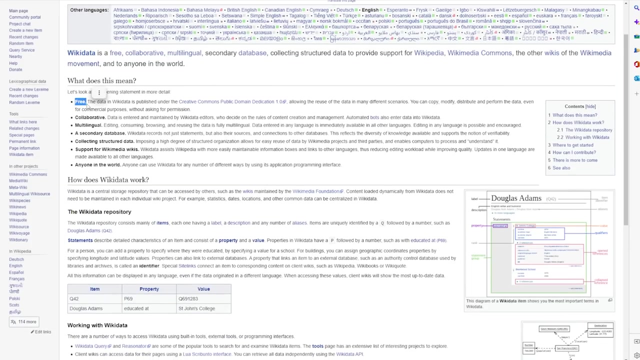 out there people could download for developers. the Google knowledge graph API is something that then people can look at. there's also various open source knowledge graphs available, as a Wikipedia has one. it's called wiki data and it's what they use to manage all the structured information they have. so you know when you go on a Wikipedia article. 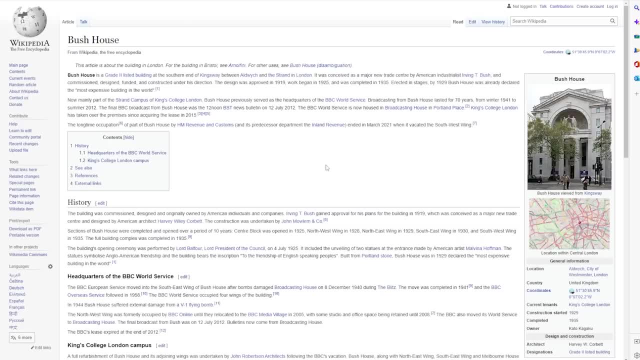 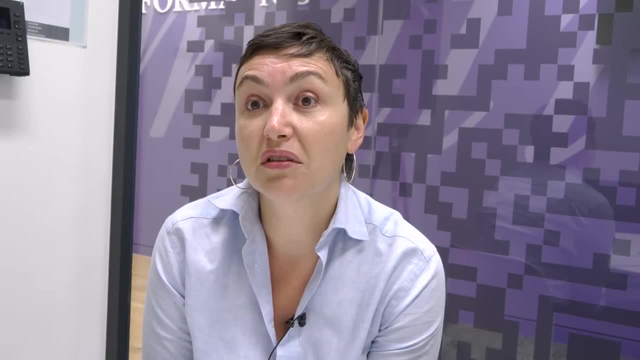 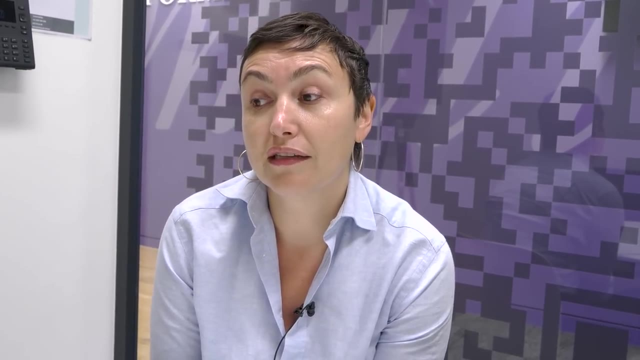 and on the right hand side you see what they call an info box- Bush house. go Wikipedia and then you'll see that comes from a knowledge graph that is publicly available and people can download it. it's quite big but at the same time you have lots of information that you can play with and I don't know train neural.